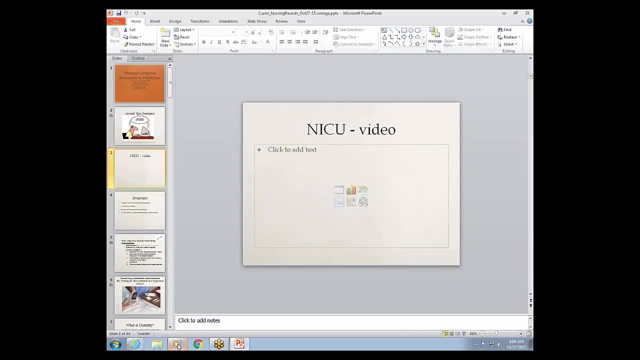 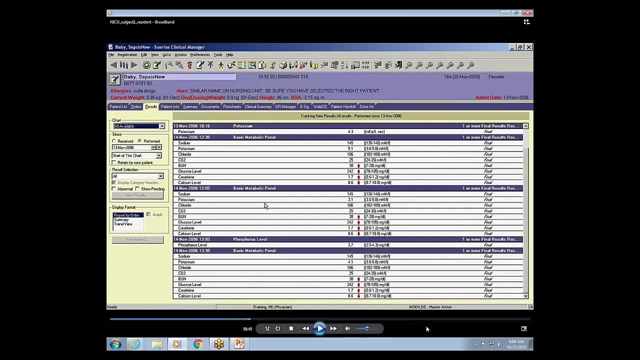 I'm going to quickly show you a little video that is an example of. this is part of a study we did in New York looking at neonatal intensive care unit challenges with prescribing. So in this scenario we've got residents, physicians, nurse practitioners in this instance. 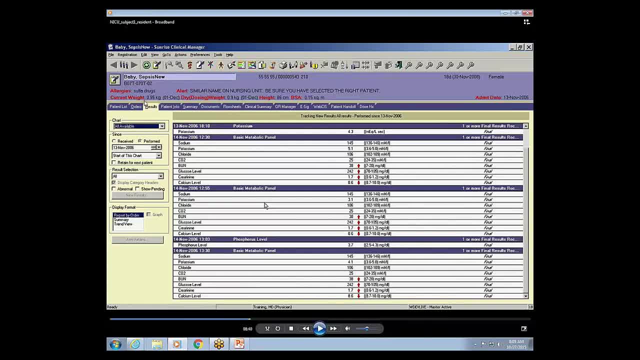 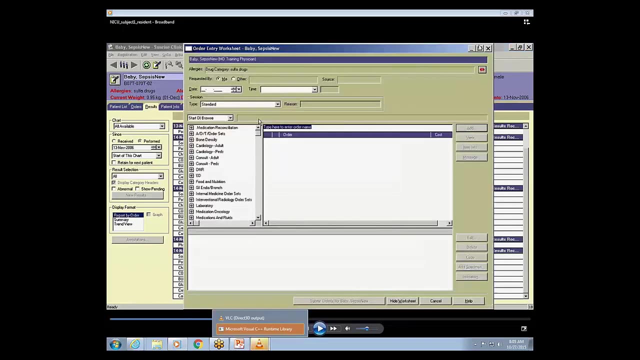 it's a resident. We have a development system, so this isn't a real person. I can hear you on your microphone. Oh, it's, it's. I hadn't hit play yet seems to be playing without playing it. 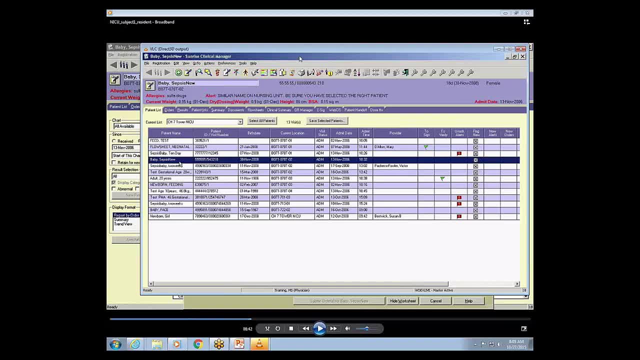 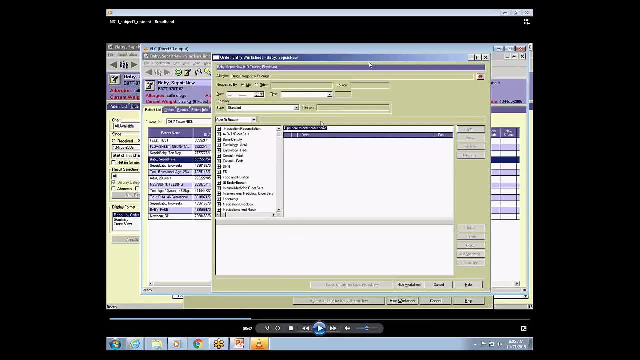 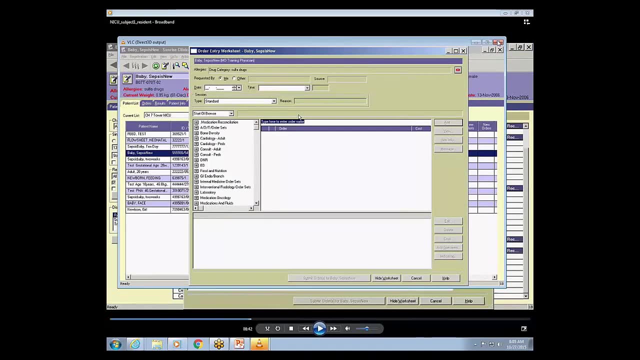 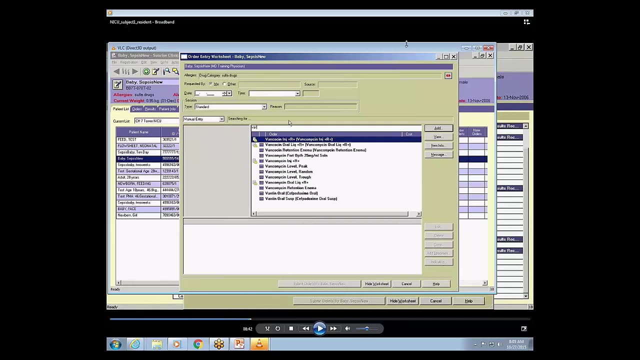 Stupid computers. yeah, Hang on, I'm going to shut this one. Give me a second here, Direct 3D, And it won't shut. Give me a sec. Okay, Okay, Okay, Instead, we're going to go for this one. 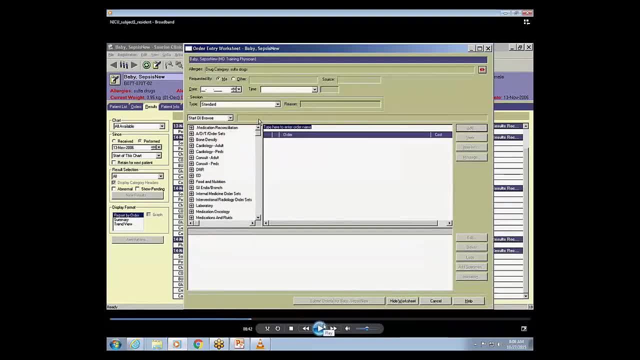 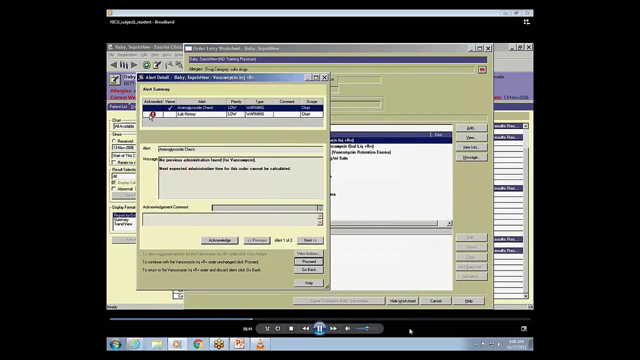 So this is an instance of we did usability testing with clinicians who were doing prescribing, looking at the user interface design and examining where a person was confused by the user interface design. So this is a resident physician trying to do an order. Okay, 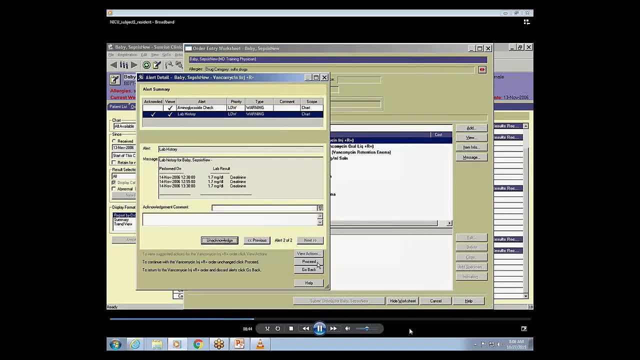 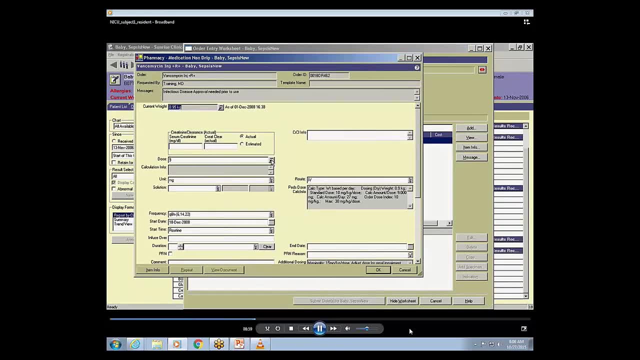 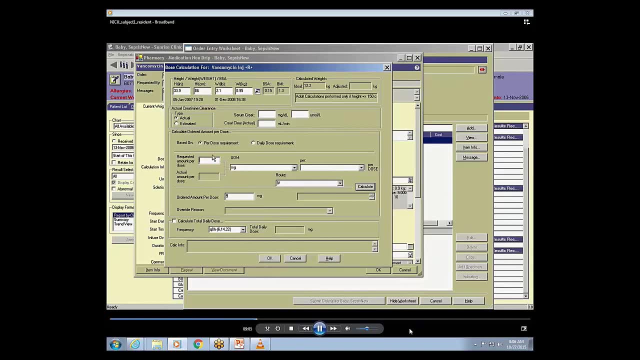 So what do you think of the how this computer system looks? It looks complex, It's really busy. It's got lots of choices in it, Lots of windows. We've given this physician a specific scenario where they're instructed on which data to enter. 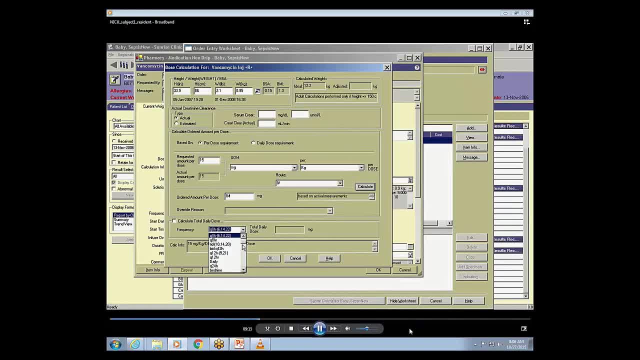 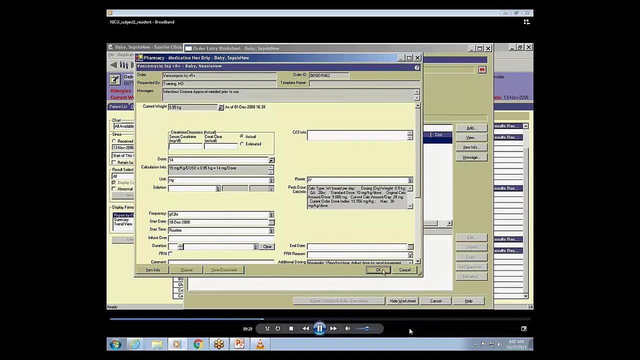 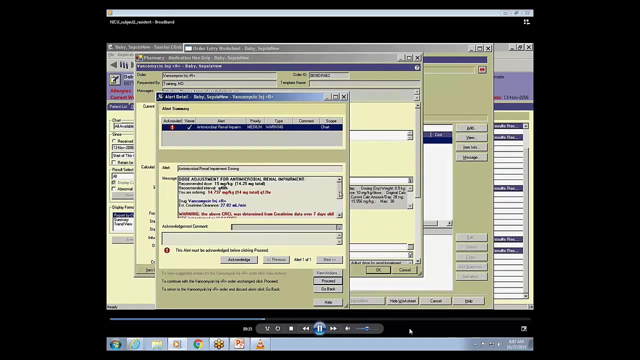 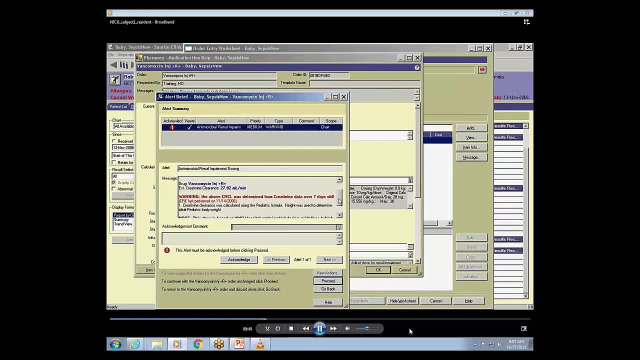 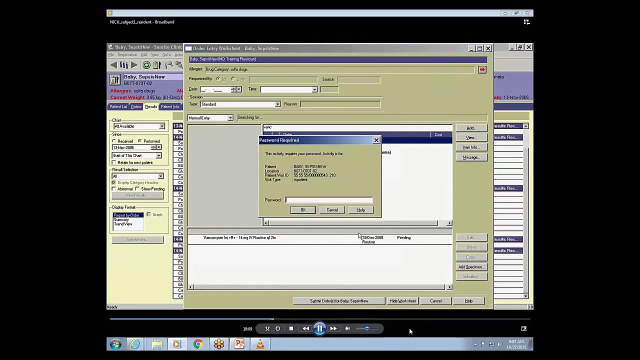 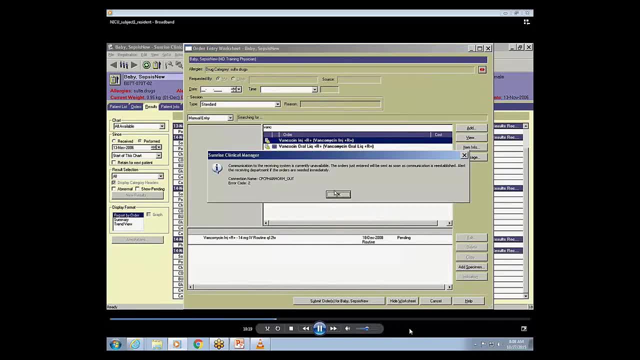 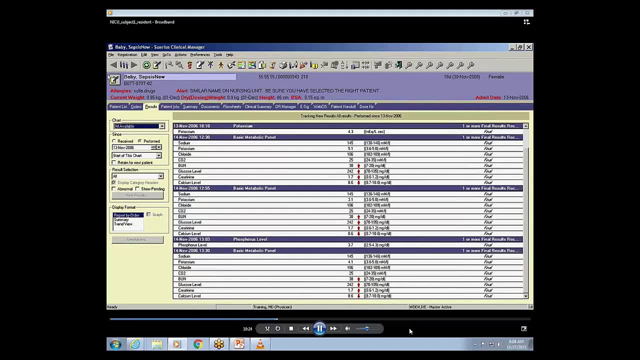 time. do you think he actually spent thinking about what the words actually said? very little, it's kind of skipping through things, and this is really really common at the point of care, when you have a system that's designed and is very complex, so people become automatic. how many of you have actually driven? 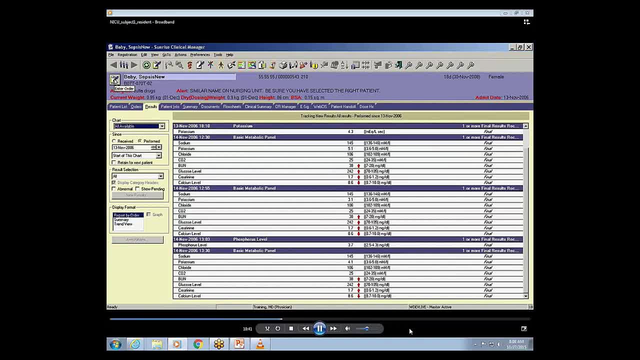 home or to work and not actually paid, not recognized that actually, how you got there? anybody done that? yeah, this happens in computer systems as well. just going to go up a little bit here, going to make another order. I want to point out that this is a fake patient. 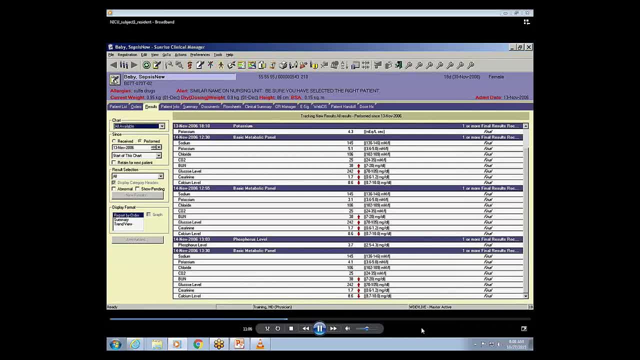 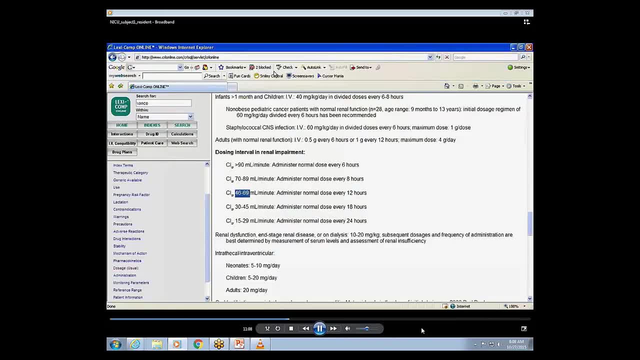 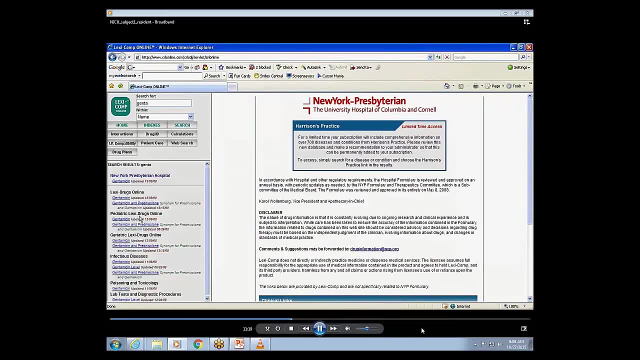 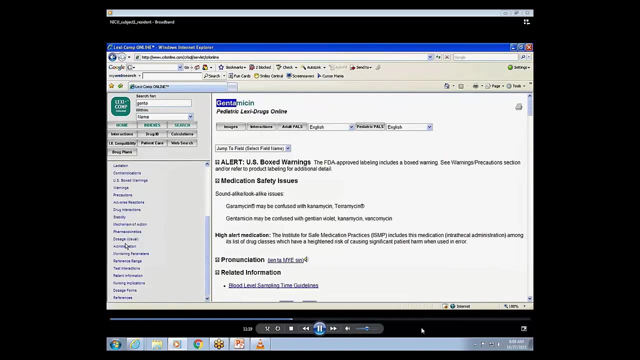 so we just called it baby with sepsis new. this is a neonatal intensive care unit context and so he doesn't even trust the prescription that's in the computer system. he has to go out and double check it and verify it. this is a big problem with your computer system. if the automatic automatic dosage 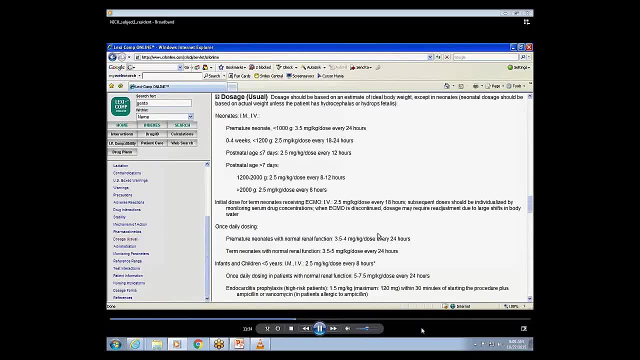 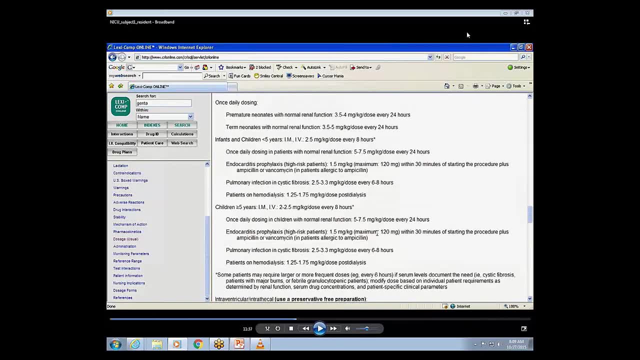 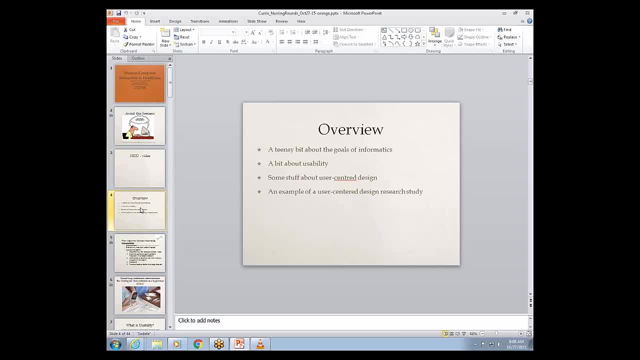 isn't trusted by your clinician, so I'm not going to go through this in any more detail. this episode was about 45 minute interaction with the end user and what we often do is we give people a series of steps and we sit back and say, uh-huh, uh-huh, and now what are you doing? 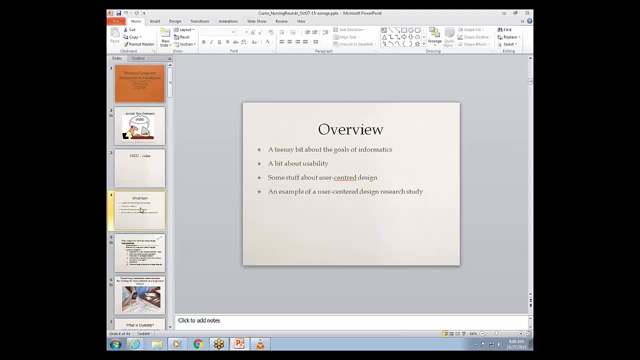 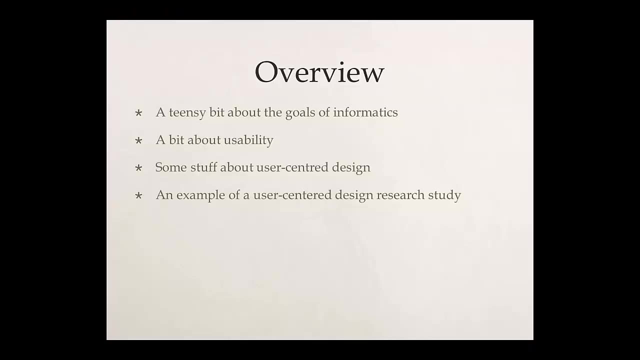 and now, what are you doing? and this is a think aloud protocol. then we take these recordings and we code them in detail, looking for a number of different things, and I'm going to talk a little bit about those right now. so today I'm going to talk a very teensy, teensy bit about the goals of informatics, a little bit about 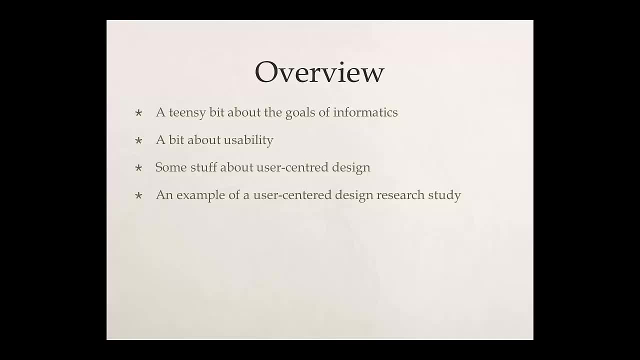 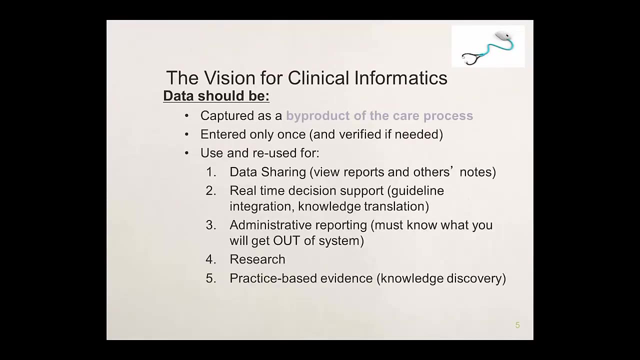 usability, some stuff about user centered design, and then I'll give you an example of a user centered design research study that we have completed the first phase of and we're seeking money for the next phase. so the overarching vision for clinical informatics is that data should be captured as a byproduct. 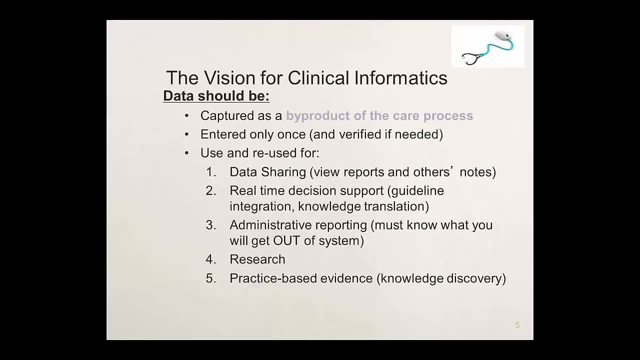 of the care process. so how do we automatically dump those EKG readings into the clinical chart or how do we capture information? so we wanted to navigate to the data. the data would be entered only once, verified if needed, and then reused and reused for data sharing, real-time decision. 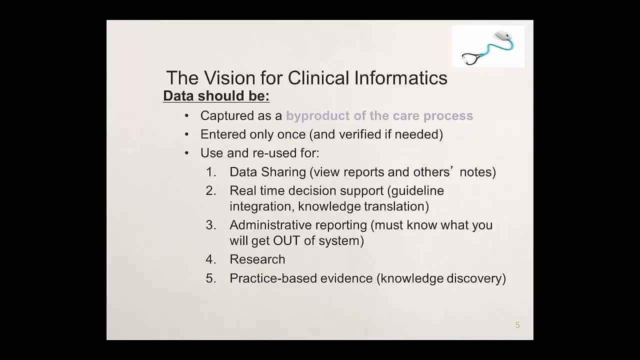 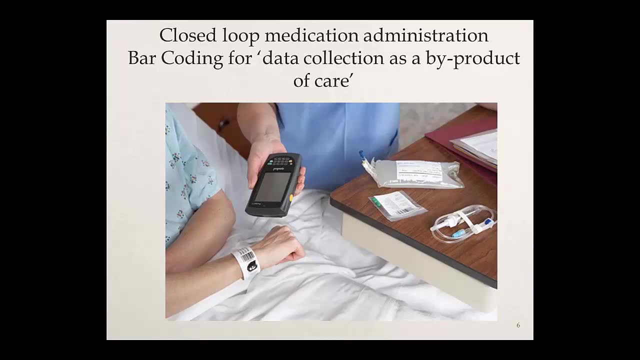 support administrative reporting, research and then practice based evidence, so discovering knowledge from the what the notes have been documented, the. an example of data collection as a byproduct of clinical, as a byproduct of the care process, is barcoding, and this is a closed-loop medication. has anybody in the room here done closed-loop barcoding for? yeah, in. 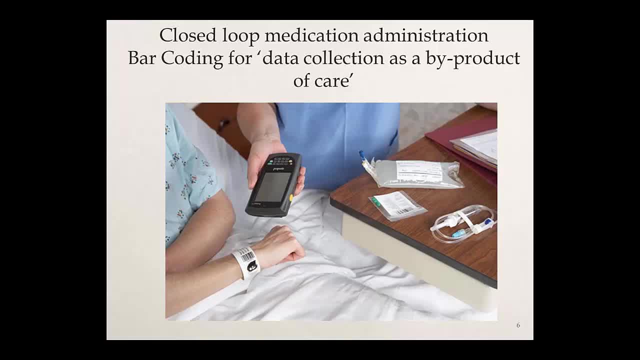 which context and in which setting in the us. yeah, how'd you like it? I loved it, and so we have lots of good evidence that it can actually reduce a whole bunch of errors. if you look at what happens here, the nurse has the barcode machine. it scans the patient's ID, verifies that it's the right patient. then 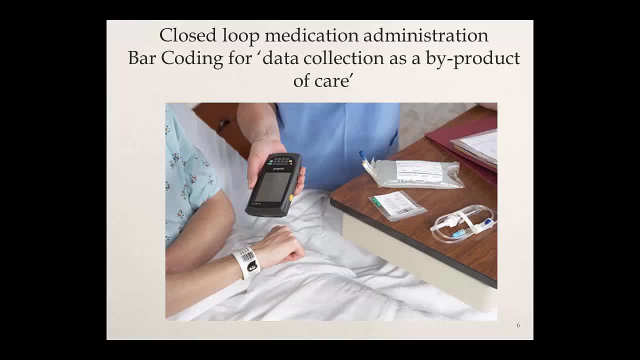 the nurse can scan the medications, verify that they're at the the right medication for that patient and tap on you. yes, this is a bit medication I'm giving, so it actually documents the time, it timestamps when the medication is given, and so this is definitely going to be. 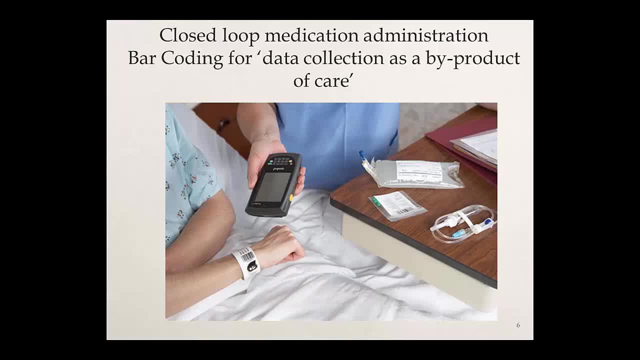 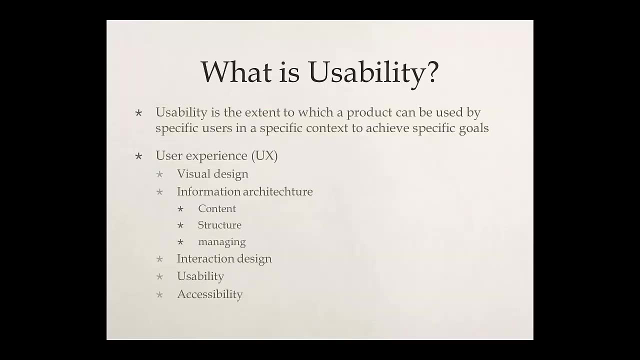 deployed it at Vancouver Coastal Health and at Providence health care and at children's and women's when they roll out the clinical information system over the next few years. so I want to talk a little bit about you. usability: so this is a concept. it's the extent to which a product can be used by. 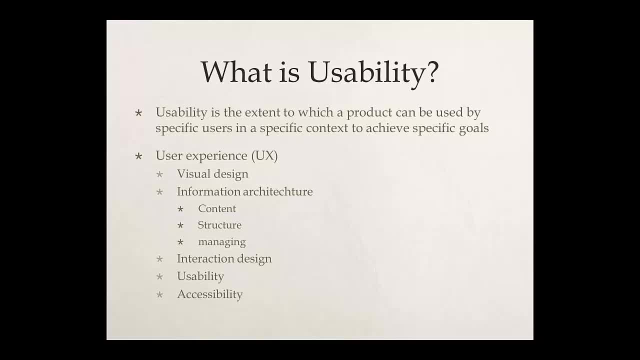 specific users in a specific context to achieve specific goals. we call this field UX or the user experience. so we're looking at a whole group of activities. we actually have some experts in human-computer interaction at a UBC in many different departments, and what we look at is: what's the visual? 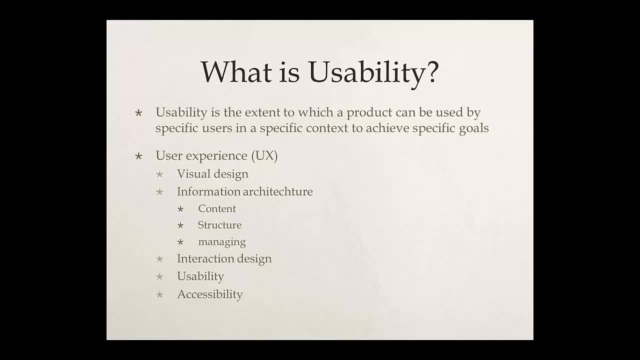 design. we also look at what's the information architecture. so how is the back end of the system structured so that the data that you're either seeing or entering are automatically captured for reuse, so we can reuse it by sharing a screen so I can see the vitals that have trended over the last several hours? 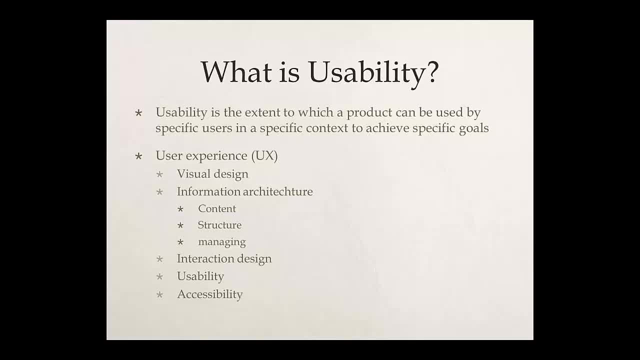 or days or months, depending on your context. we want to look at the, the structure and the management of it, so usually we need people who are managing the databases to keep things well organized. we can look at interaction design. so how do humans interact with computers? one of the things that we can 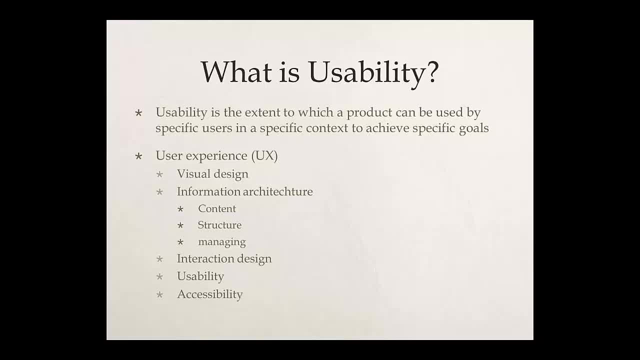 do is eye tracking, so there are people trying to look at using retinal scan for accessing the computer system instead of having to type in your password. when you're a clinician working in practice, when might that be a good idea? yeah, so for infection control reasons? yes and so. 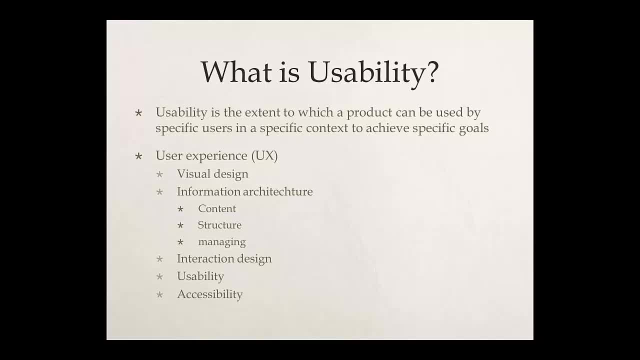 what sort of other technology might we want to enable if we've got dirty hands and can't touch the computer voice? so speech recognition systems are starting to be deployed in health care and we're looking at how can we effectively automatically capture the data at the point of care. then we look at usability. I'll talk a little bit more. 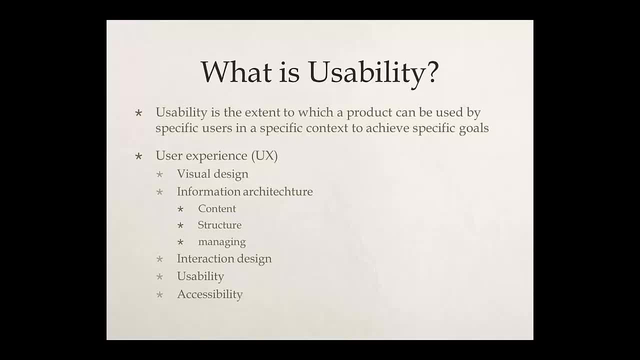 about it and then this idea about accessibility. there's a whole other topic area that we call the digital divide wide, and this is the idea that if someone doesn't have access to the computer system- and health care is deployed ubiquitously by Computer Systems- that we may be further alienating individuals who are already. 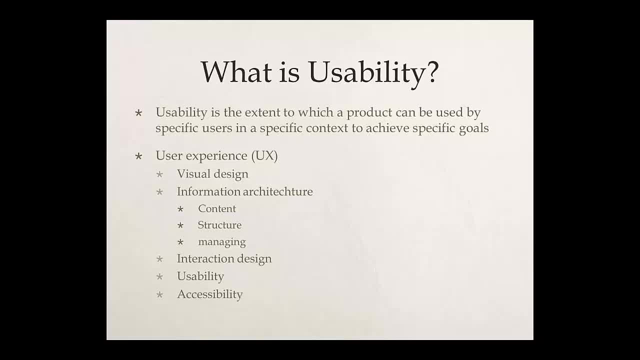 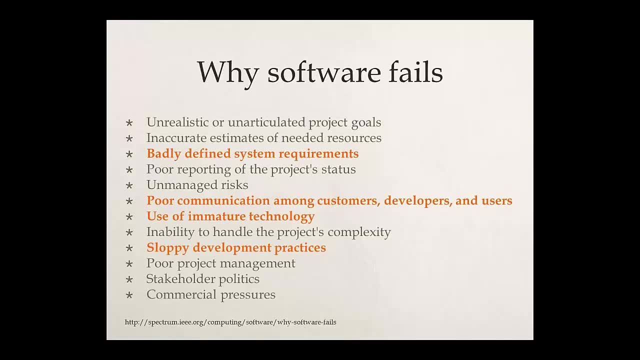 marginalized, and so we have to be mindful of that. so there's a whole list of reasons why software fails. if you- they suggest that if you software fail, endena fix something before it's deployed. it costs you a dollar per problem If you fail to fix that. 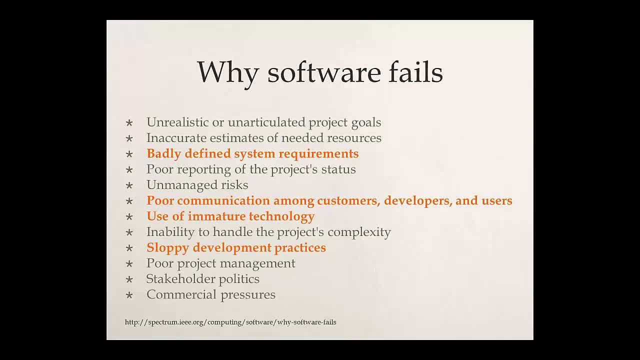 problem. it can be a thousand dollars to ten thousand dollars to a hundred thousand dollars, depending on how complex the problem is, to fix it after you've launched it. So the goal of the whole UX, or user-centered design, initiative is to make sure that we have activities. 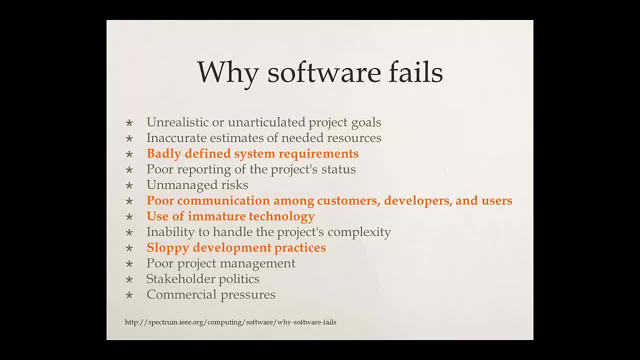 in place to test it with end users before we launch a full product. Then we can capture different things. These are probably usability issues, badly defined system requirements. So system requirements is when we're trying to design something, we look at what are the functions that? 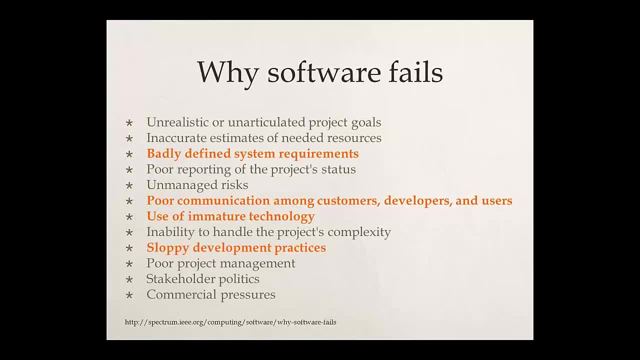 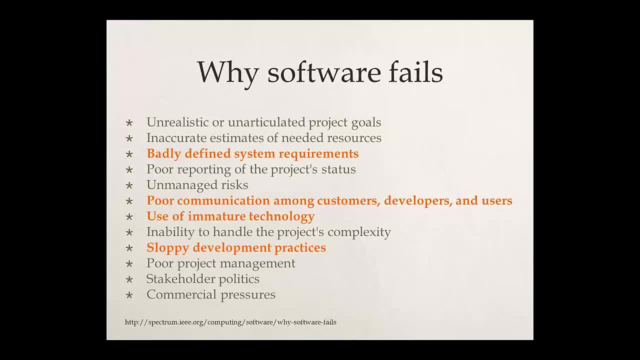 among customers, developers and users. Use of immature technology, so launching something before it's actually fully functional. You may be living through that in some instances of products that you're buying. It's actually considered standard practice in some areas and people try to do it in healthcare. It's not best practice in healthcare. 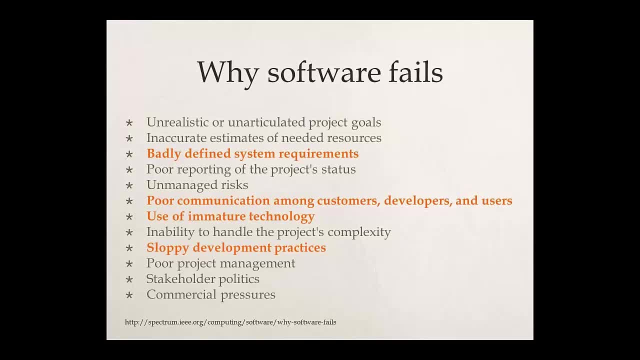 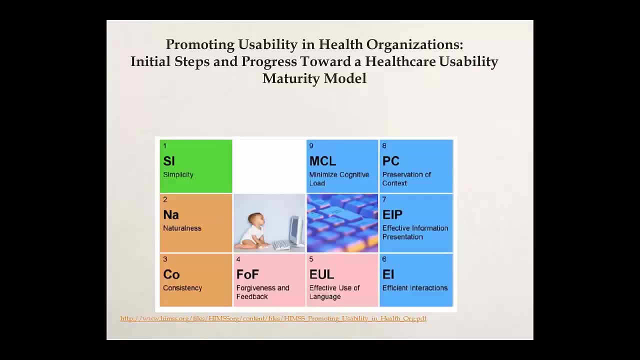 And then sloppy development practices, So not really figuring out the logic and doing actual testing before you launch something. This has been such a big problem that the Health Information Management Systems Organization has actually launched a healthcare usability maturity model. So if you're in a, the goals are to make the software. 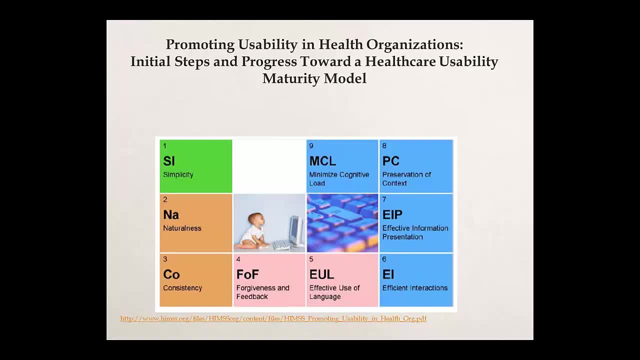 appear simple. How many of you have an iPhone? Almost everyone. Who's got a Blackberry yet Android Couple Androids. So when you first bought your iPhone, how was it compared to that flip phone or that chocolate bar phone you had before? It was like super awesome, 10 stars, 12 stars, if you could. 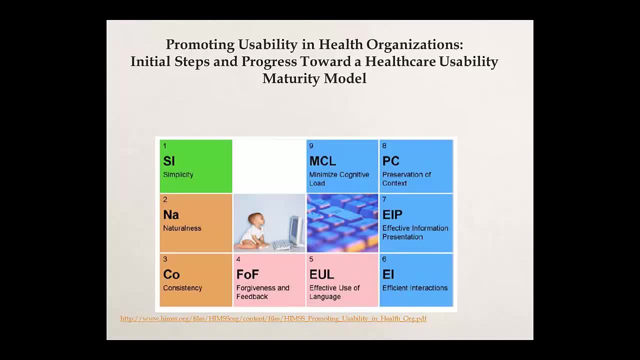 No, Except for one individual who hates it. Okay, So the idea is the amount of years. they didn't launch the iPhone until 2009.. They had the iWatch in production for almost 10 years and it wasn't launched until last year. So they- Apple- will not. launch product before it's had massive development and other things, Because it was launched in 2009,. it was the first iPhone to launch and it was this amazing product that was launched in 2009.. And so they- Apple- will not launch a product before it's had massive development and other things, Because they don't have, I think, a large number of users that are very, very good at having the technology to eat it. So they're going to have a solution for And to have a solution that's really important. So they're going to have a solution. 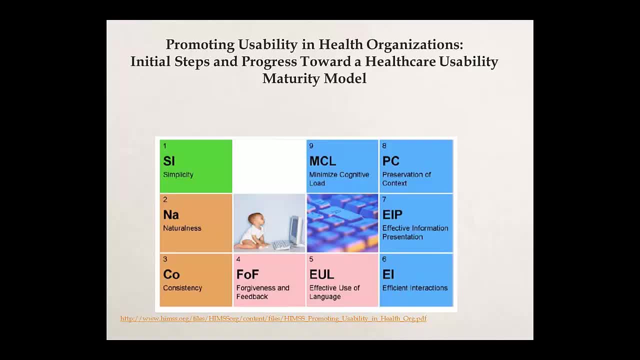 within that product and it's going to have a solution. that would be, I think, a solution that's really important. I think it's very important- maximum amount of usability testing, but we're not doing that in healthcare. We want to strive for simplicity. 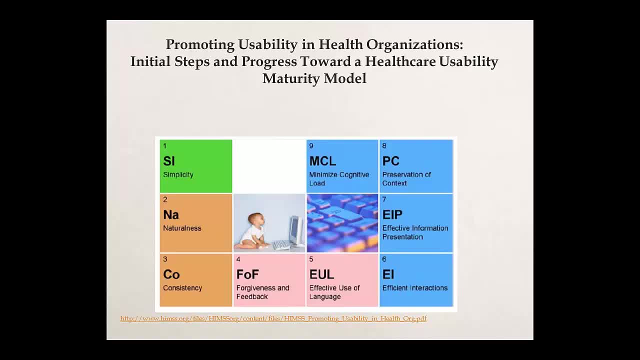 We want to minimize the cognitive load. We want to preserve the context and in healthcare that's the knowing who your patient is and where that patient is in their care continuum. We want it to be natural, as natural as possible in the context of healthcare. 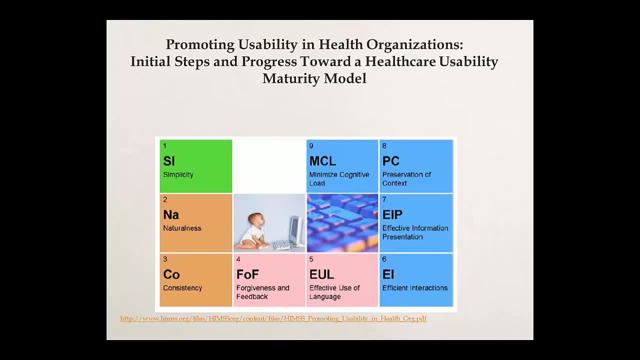 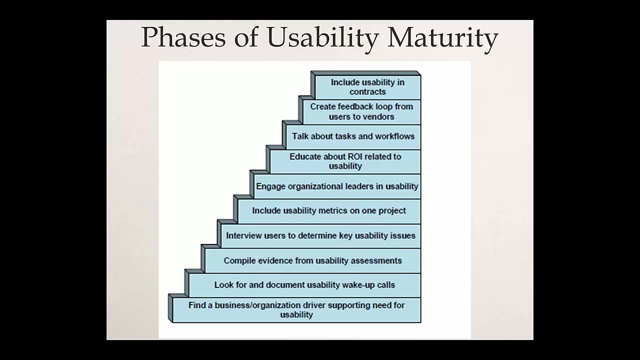 We want consistency, We want forgiveness and free feedback, Effective use of language, effective information presentation, efficient interactions. So these are all, as they say, end of the rainbow dreams, and we ain't there yet. But the Health Information Management System Society has suggested that organizations need: 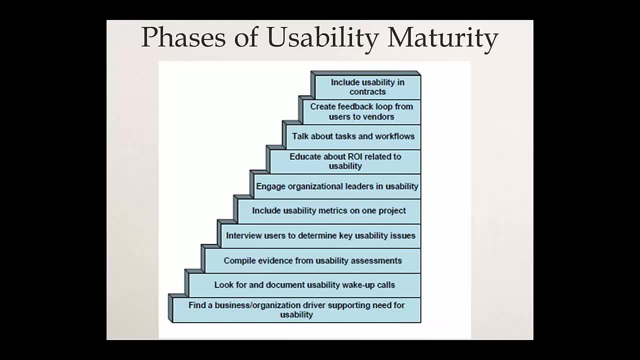 to figure out how to have usability Be part of their deployment and development process. So, from the bottom here, anybody, a business who's down here, there might be someone who is supporting the need for usability. There might be usability wake-up calls. 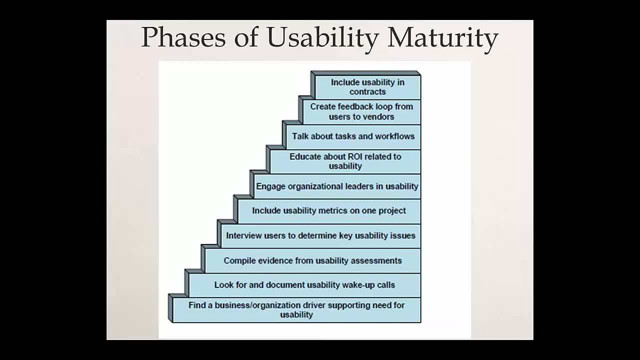 In healthcare. what does that end up? as If you've got a bad user interface design, Safety. So what might happen? Errors, And then what might happen? Someone dies, Yeah, And we've got evidence of this. and if you're not adhering to best practices, we have evidence. 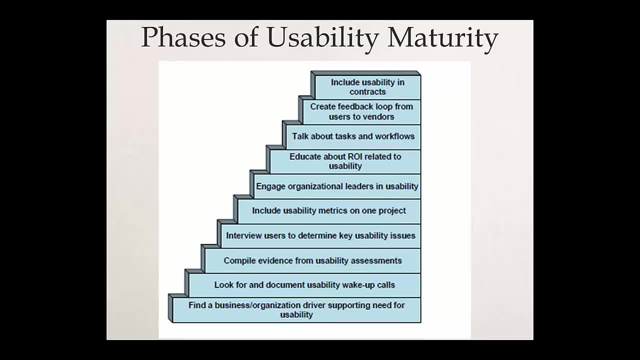 of deaths due to technology-mediated adverse events. An organization could compile evidence from usability assessments Up to the very top. Include usability in contracts. In healthcare, we're purchasing a contract with a company that provides a software. It's highly unusual for a healthcare organization to build their own electronic health record. 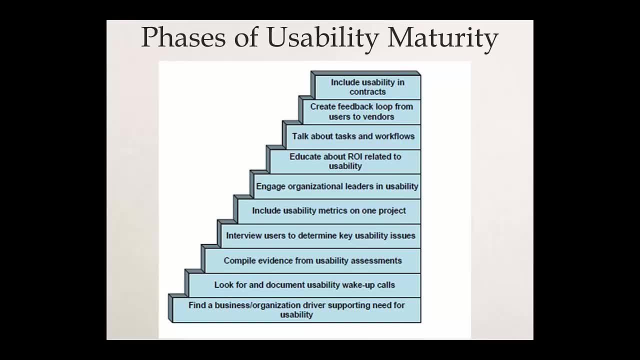 And so an organization is fully mature if they make sure that usability is included in the contract. Not always the case. Organizations don't necessarily know the implications. They presume that if a company is selling you something that all of the safety tick boxes have been checked. 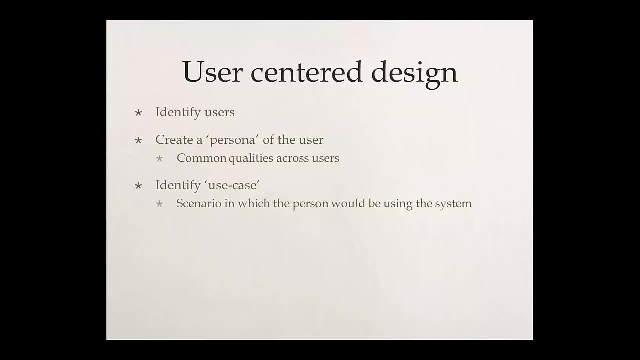 It ain't so. So with user-centered design, we want to figure out who the users are. We typically create a persona of the user, So this is like a base case of a person to get a sense of who's the typical person that's. 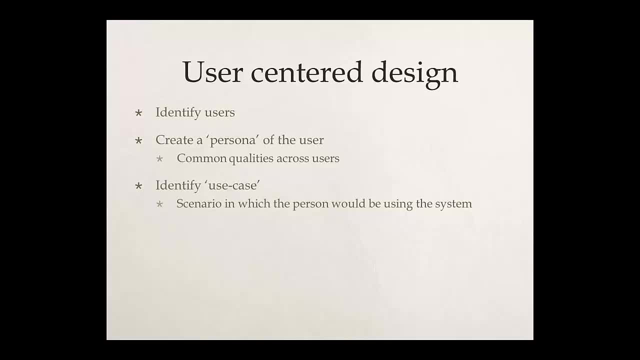 going to use this system. We look for common qualities across users. Then we identify this thing called a use case, and this is a scenario in which the person would be using the system Now flinging these words at you because it's important for nurses to not sit back. 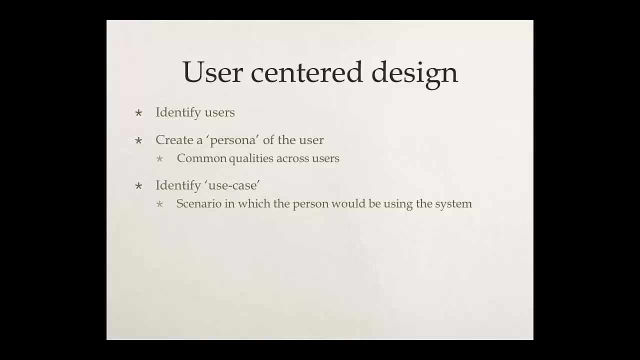 and not know some of these words. because what happens? there's a power gradient between the software engineers and the healthcare providers And if they don't know some of these words, they're not going to be able to use them. And if you ask somebody, well, what's the use case? 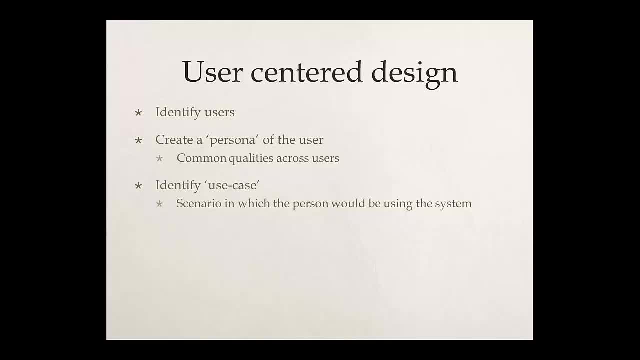 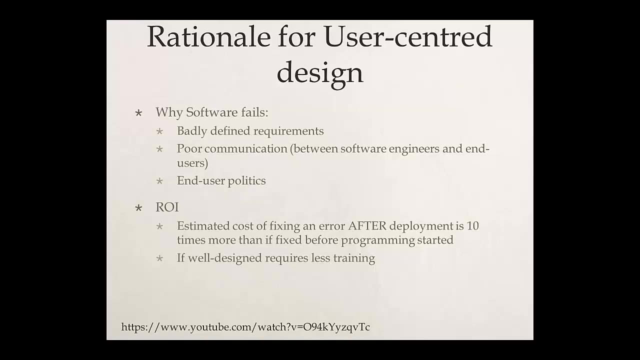 That's their lingo- for a scenario in which a person would be using the system And they'll realize: oh, you have some knowledge about this and you're going to maybe hold them accountable. I've mentioned why software fails. There's a YouTube video here and I can post these slides, if you want, for looking at a. 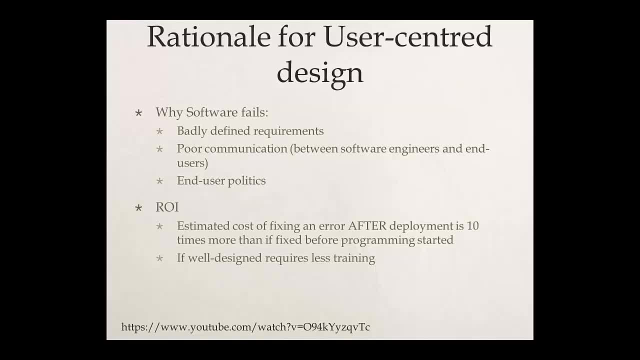 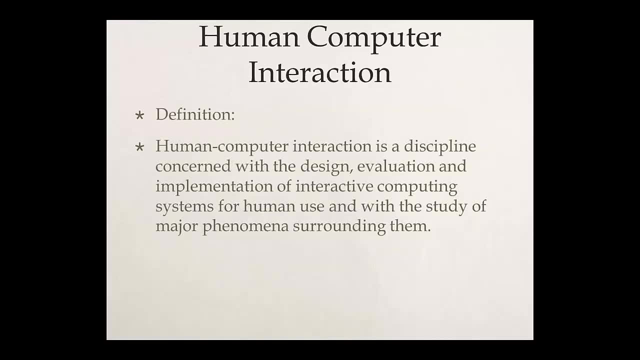 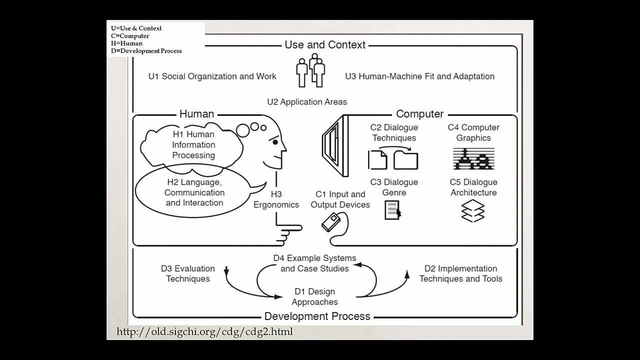 return on investment, But the cost of fixing an error after deployment is 10 times more than if fixed before the programming started. Human-computer interaction: It's a discipline concerned with the design, evaluation and implementation of interactive computing systems for human use, with the study of major phenomena surrounding them. 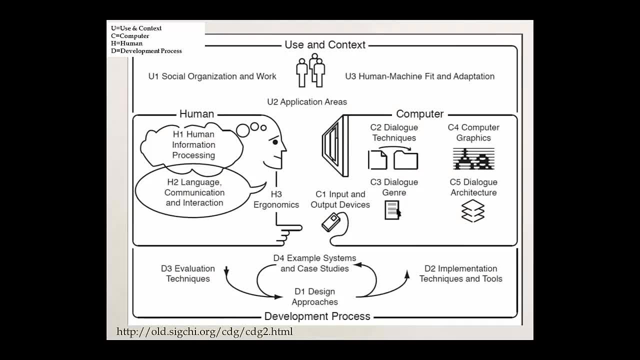 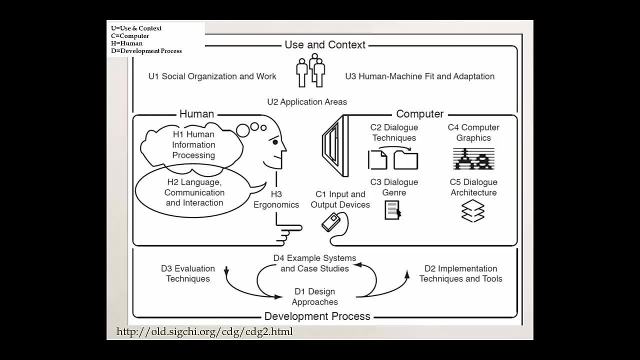 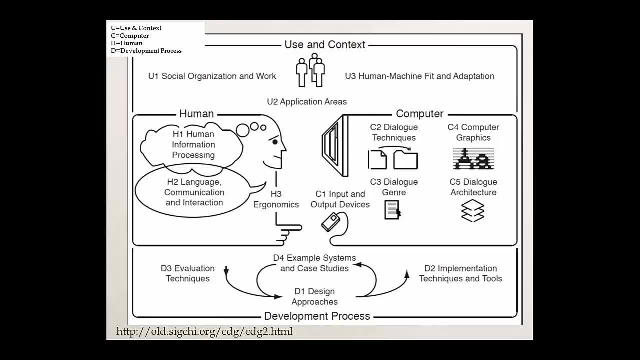 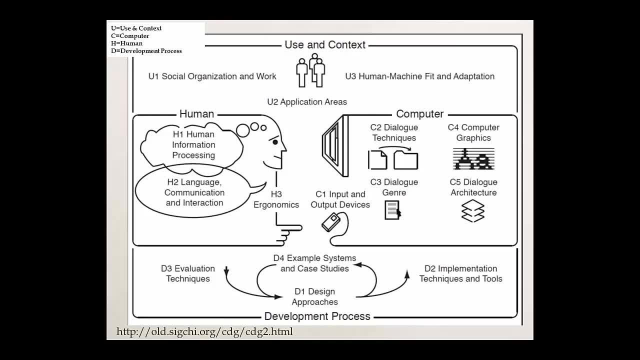 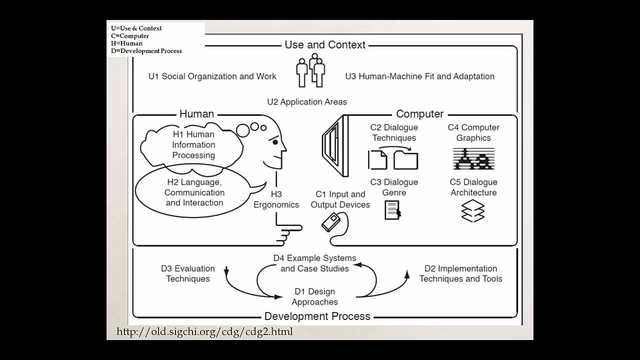 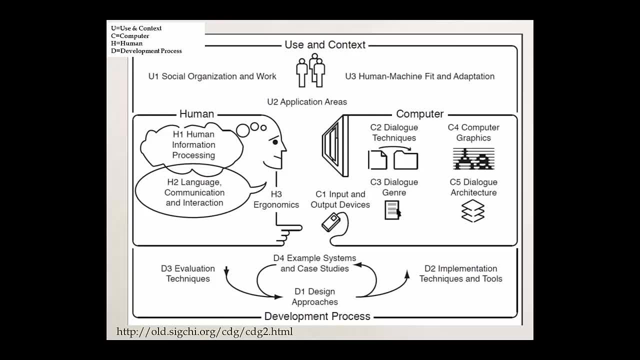 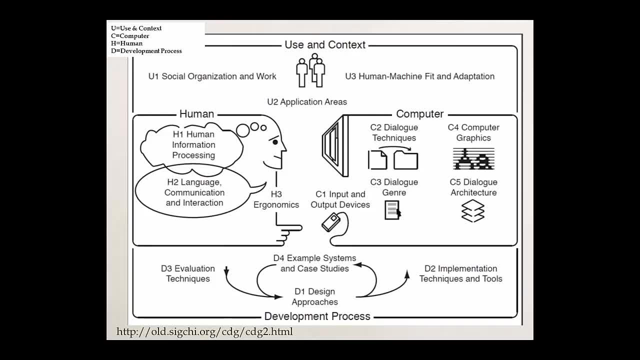 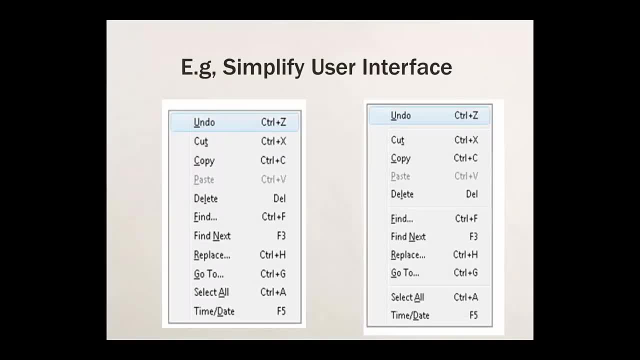 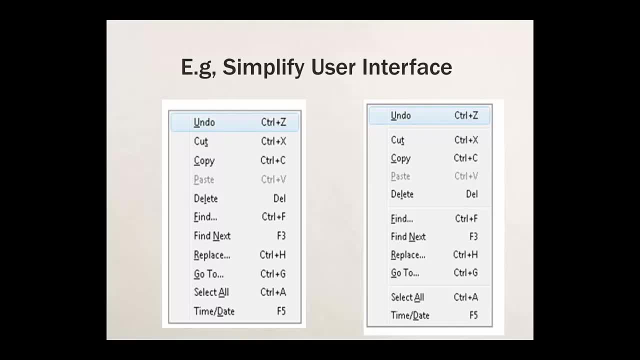 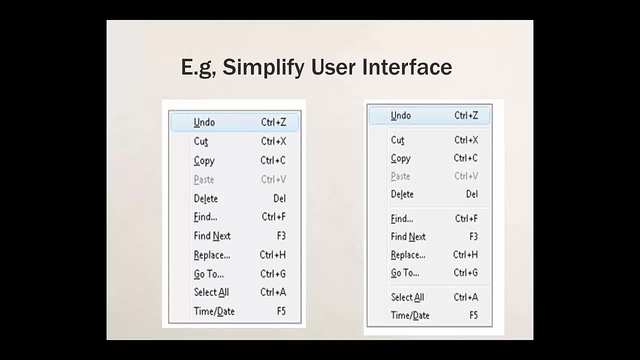 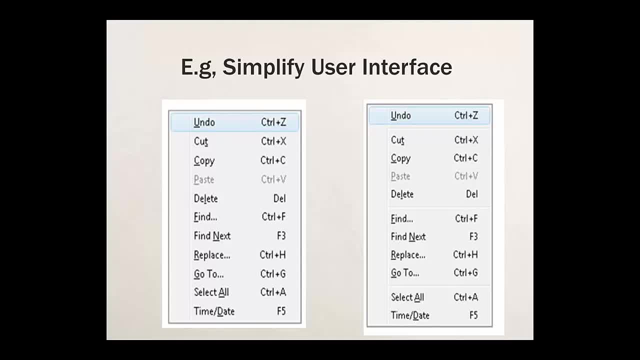 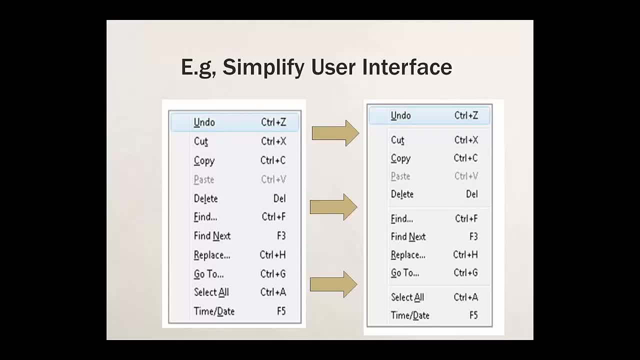 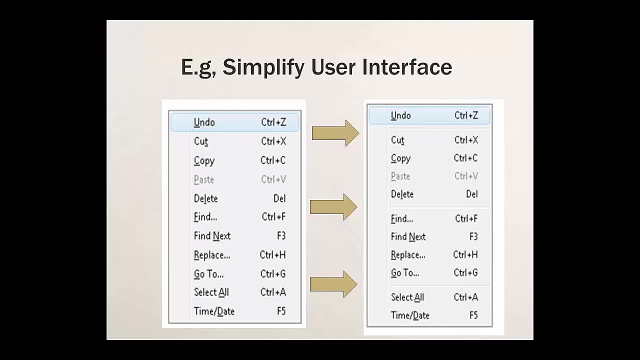 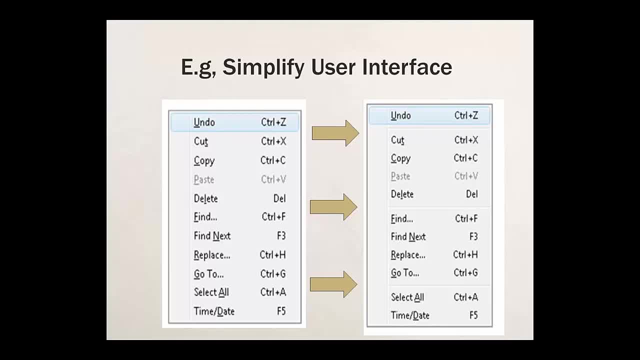 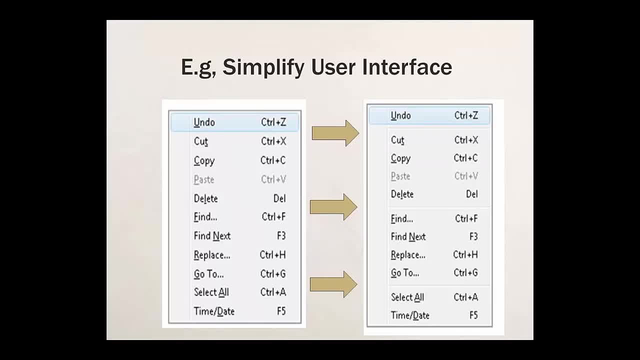 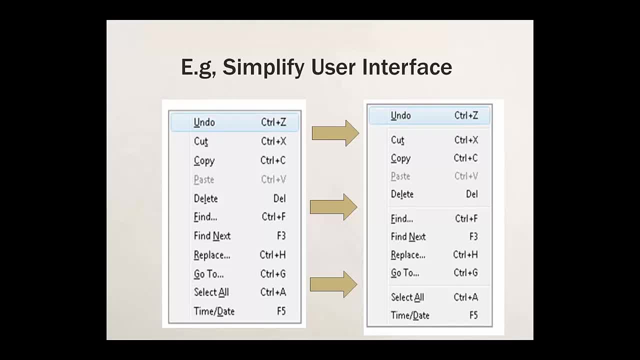 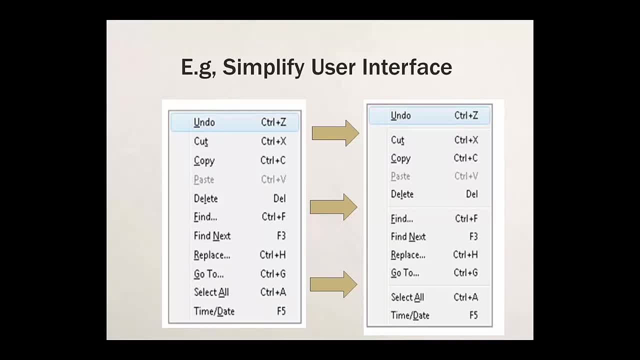 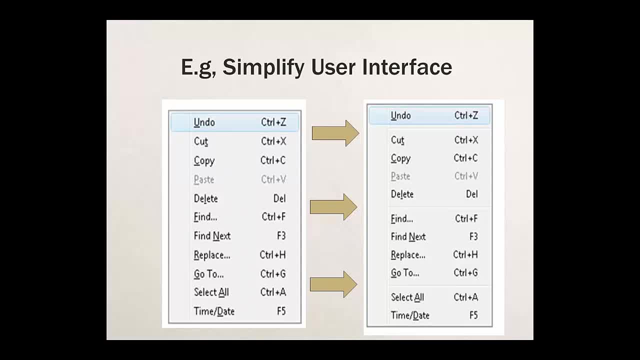 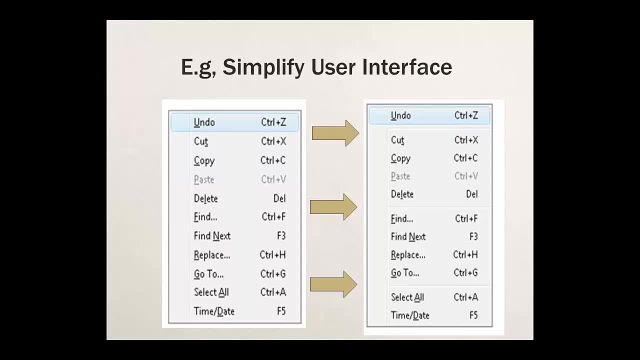 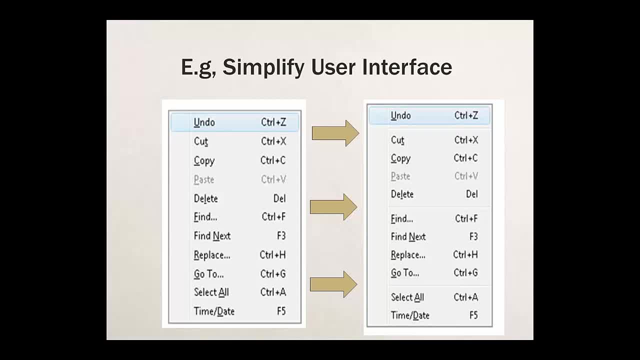 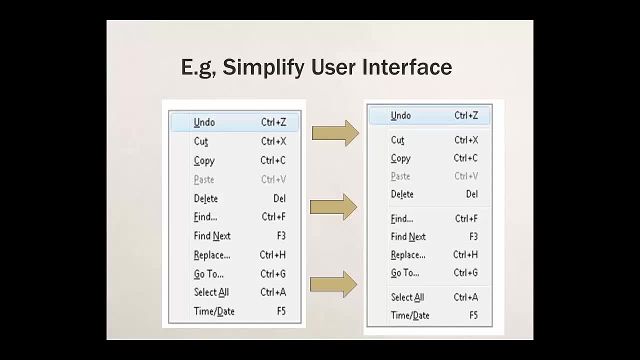 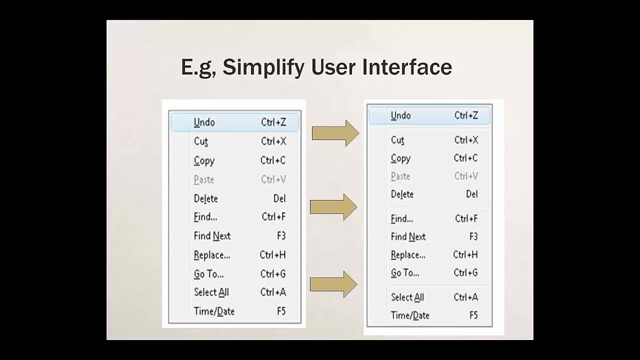 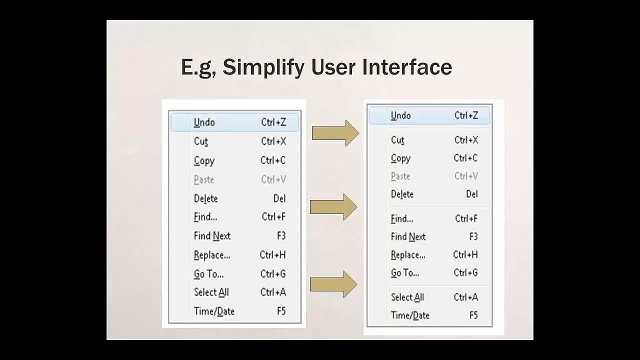 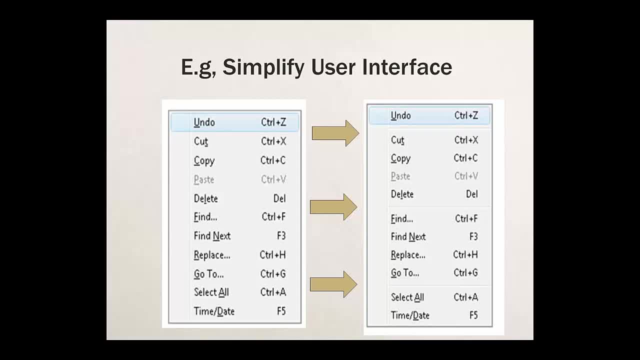 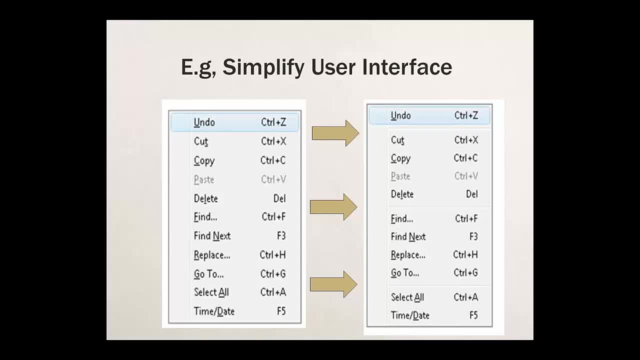 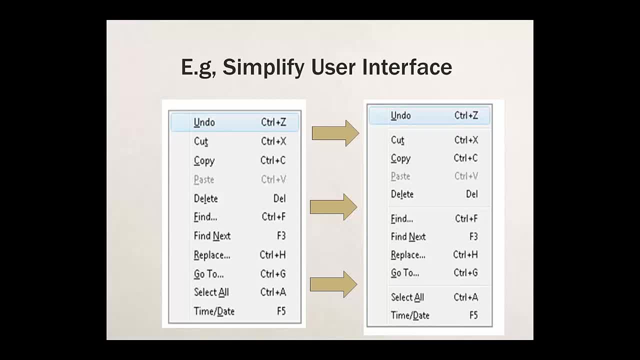 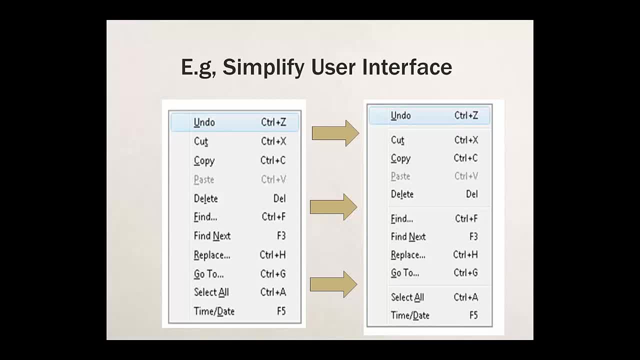 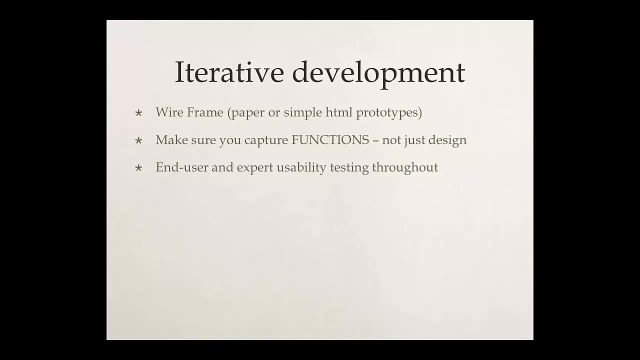 We also use an iterative development process. I'm going to give you, I'll show you- an example of how we've used wire framing, which is a process where we have a fake user interface that people can click through. It doesn't deposit any data into a database, so it's easily morphable and fixable. 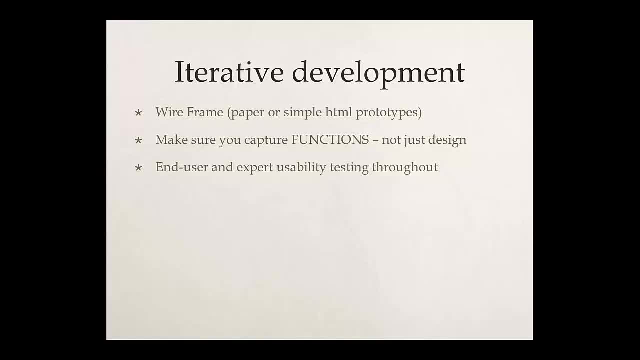 And the goal to use. most organizations that put any money into designing computer systems for their workers have spent a lot of time doing pre-prototyping and getting the understanding of the user experience. We want to make sure we capture functions, not just the design. 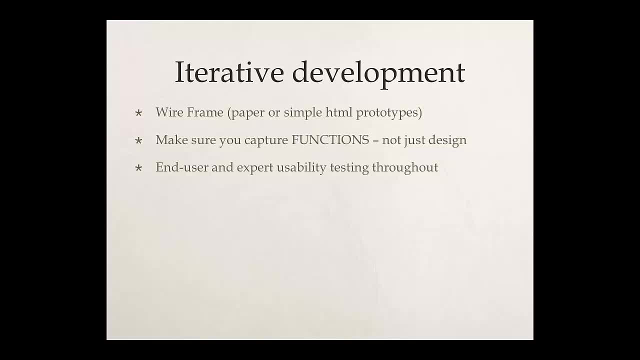 Has anybody been part of a paper prototyping or computer system development? Yeah, what have you? Oh, you're on the CST project right now and they're just using paper prototyping With In the development system, Right, Right. 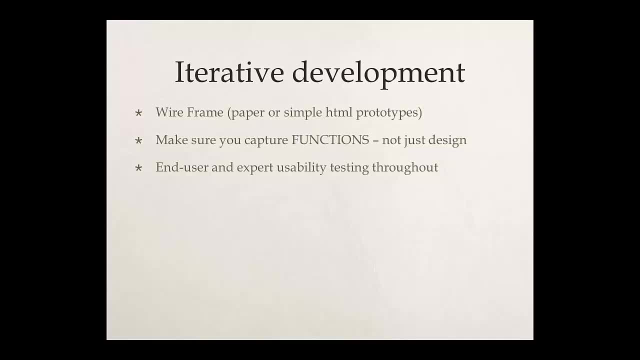 Okay, great Good, because the thing is that you have to make sure you have actual end users- naive end users- using it. Don't just ask yourselves if this is good enough. What often happens in organizations is they do what they call user acceptance. 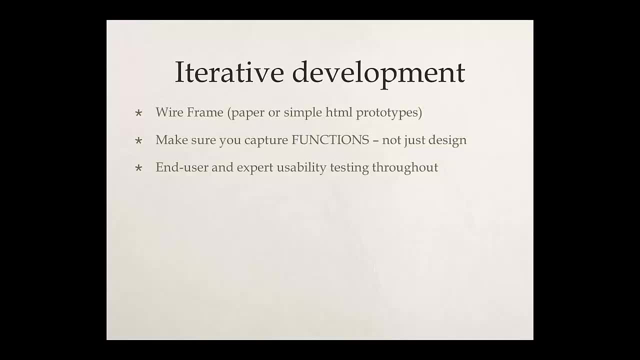 That's their evaluation mechanism is user acceptance. Instead, you need to be doing end user and expert usability testing throughout the process. So usability testing and expert evaluation could be what we call a cognitive walkthrough. Another method is a heuristic evaluation. So this is taking that persona, walking through a scenario and thinking about what are the violations to usability standards, best practices. 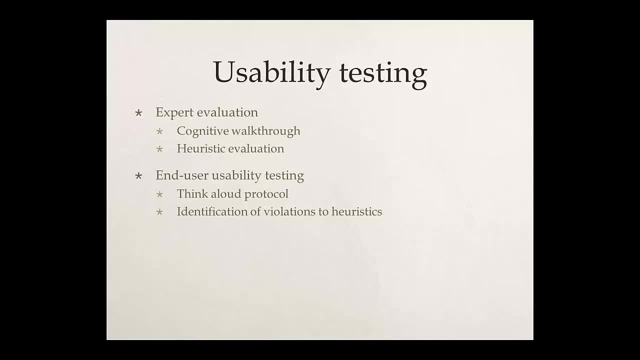 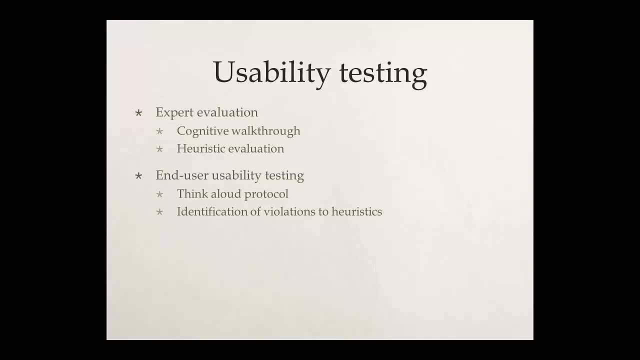 We can do end user usability testing with a think-aloud. We can do end user usability testing with a think-aloud. So the example of the video that I showed you was a think-aloud protocol or talk-aloud protocol. So we gave all the residents and nurse practitioners that were in that study the same scenario. 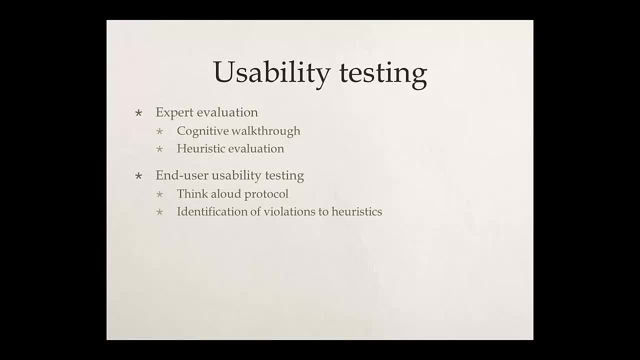 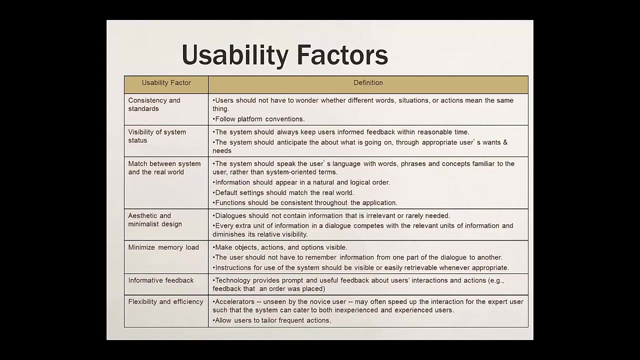 and we designed the system so it would force them to all see the same thing, And what we were able to derive from that was a lot of information about where they were skipping over things and ignoring the alerts- Very, very helpful. This is a list of these things we call usability factors or usability heuristics. 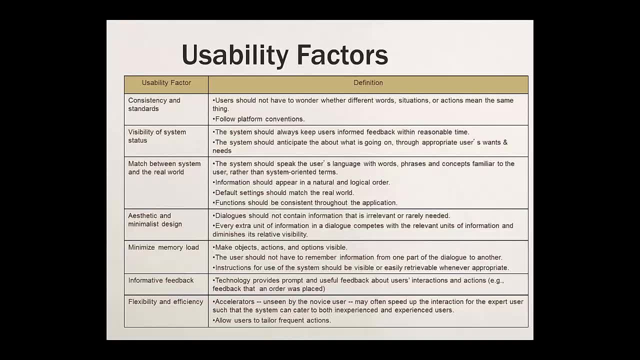 So heuristic, the modern definition of it is a rule of thumb. So these rules of thumb are many of the things that we want our computer systems to actually be achieving: Consistency and standards, Visibility of systems. Describe parts of it. Describe parts of it. 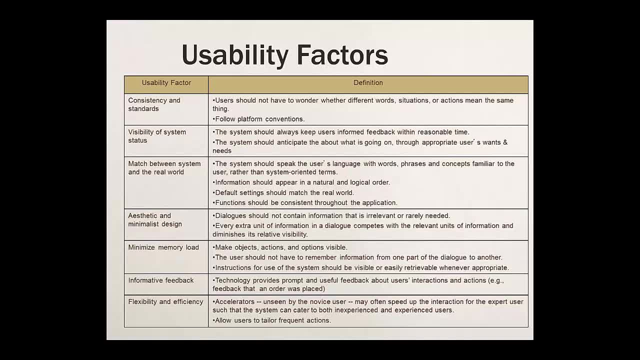 status. Can anybody think of an example of visibility of system status in a computer system? you're using right now The wheel of death. that's right, but when the wheel stops spinning, it's the wheel of life, right. So, yes, you know that. or if you're on a website, sometimes you'll 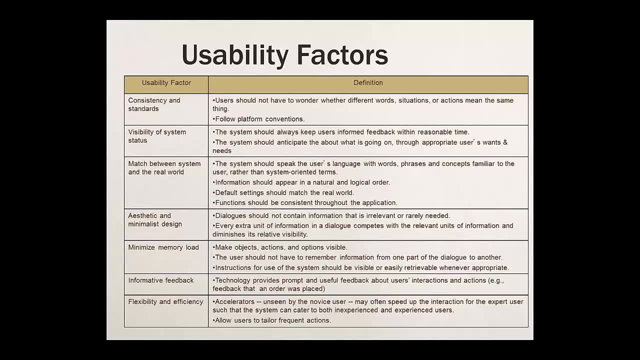 see the little cursor, Expedia. it has the little dots that are going back and forth telling you that it's still alive. That's very commonly now implemented. Ten years ago it was not the case. You would be on a website, you'd click on something. 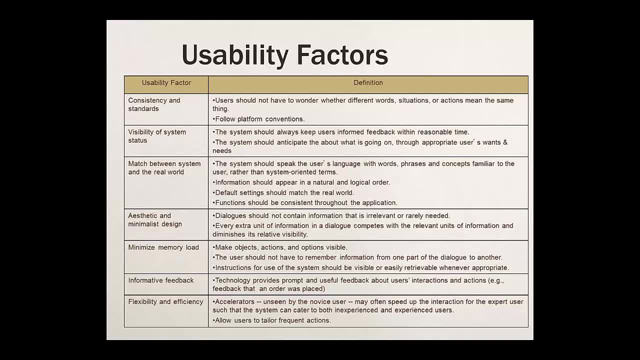 and you'd be like: did I do anything? Has anything happened there? And maybe they became creative and, instead of showing you that you're still interacting with some sort of a system by showing you something that's moving, they might actually have big font that says: 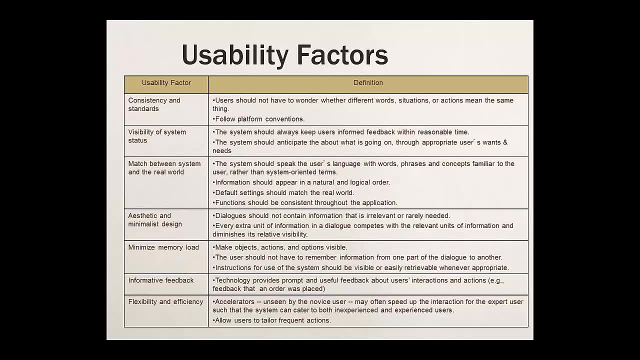 do not use the wheel of death. Click again, right, I'm thinking anybody use the RISE system for research ethics here, Yeah, match between system and real-world minimalist design, minimize memory load, informative feedback, flexibility and efficiency, And you can. 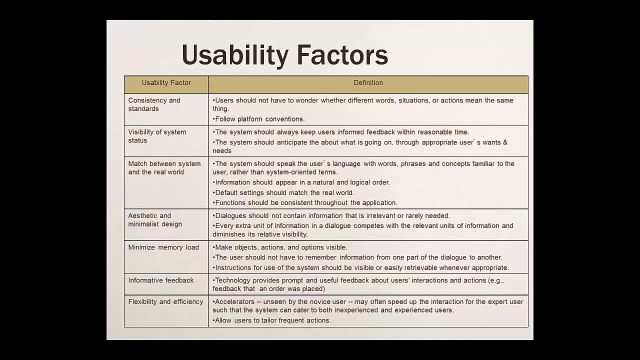 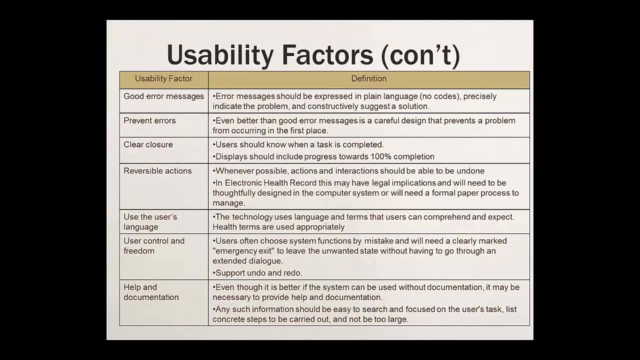 see, these are similar names to those things in the boxes from the Health Information Management System Society. There are about 14 of these right now. Good error message, clear closure. You should know when it's complete. So an example of that is like an online survey that you might do: What do you see at the 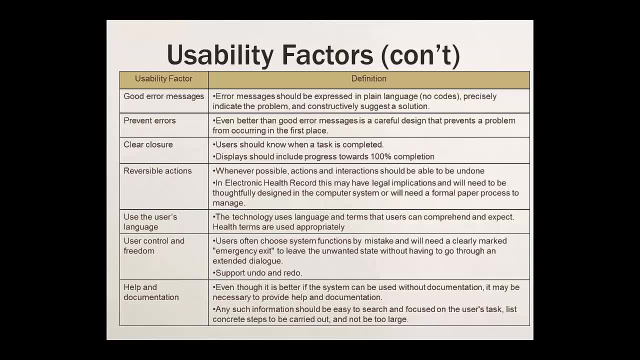 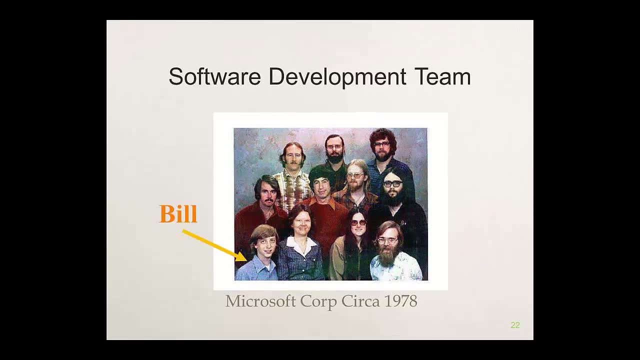 end of a survey, ideally. Yes, thank you, You know. click here to give us your email so you can enter the raffle, or whatever it says. So if we have poorly designed systems, a number of things can happen. So here's our software development team from a few years ago: The Pacific Northwest. 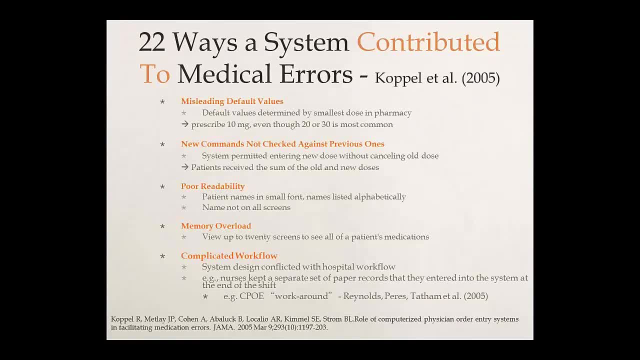 GARB and BEARDS. We've got lots of evidence of technology mediated adverse events. This study was from 2005,, published in the Journal of the American Medical Association. Misleading default values. So the default was the lowest dose, not the most common dose. 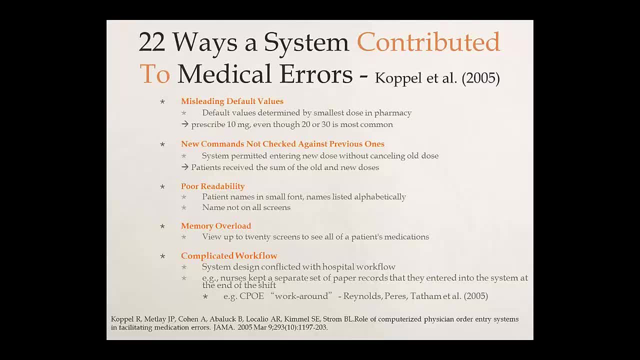 So people would just pick that. You saw how automatic that resident was with clicking through things. It's super easy to make a mistake. New commands in this system. this system has the company has been purchased by another company, so this system is retiring. But new commands, not text against previous ones. So people 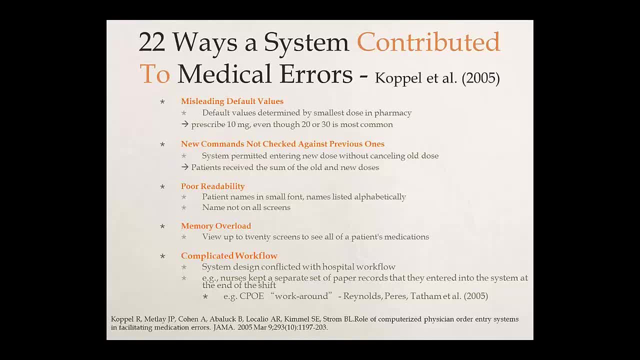 could get two orders for the same medication. Poor readability, Patient names in small font, Names listed as alphabetically Names not on all screens- Huge, huge problem, And you'll see that even in existing systems. So you need to make sure that someone's checking for these things. 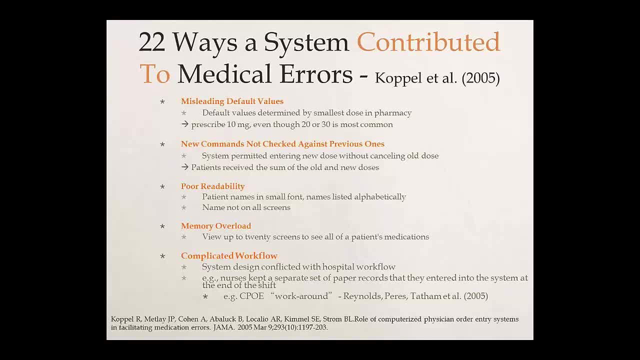 Memory overload Up to 20 screens to see all of the patient's medications. Ok, who designed that Complicated workflow? The system design conflicted with the hospital workflow. The nurses kept a separate paper record and then entered the information into the computer system at the end of the shift. this is a. there's a. 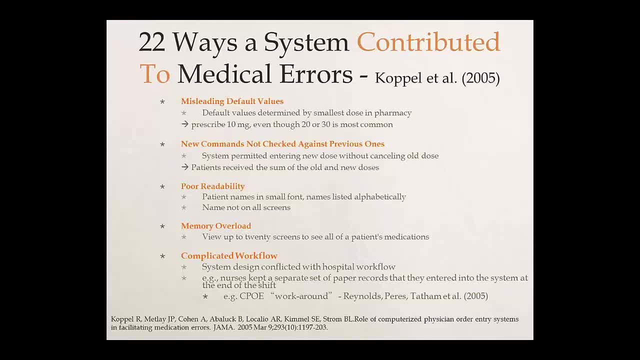 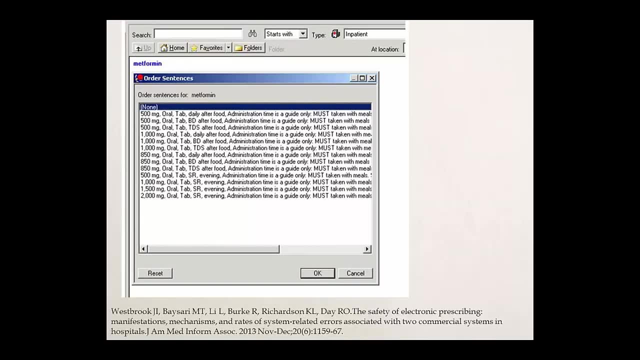 lot of evidence about workarounds, so here's some examples of some safety of electronic prescribing manifestations. a rate of system related errors associated with two commercial systems- so this is a relatively recent article- our colleagues in Australia and the- you can't read the entire sentence for each of these- 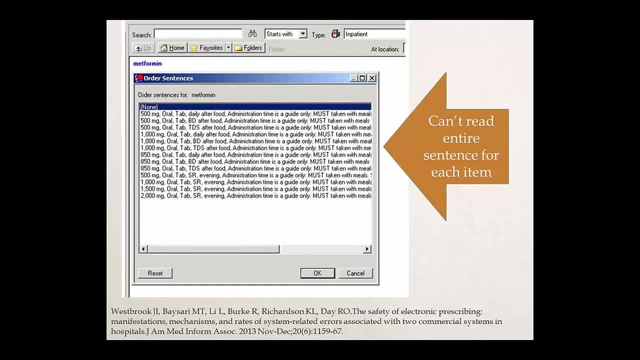 medications. so you've got metformin up here as and the case of this is hard to read. these things should be in title case. the first word is capitalized. the other words are the other letter. the first letter is capitalized, the other letters are lowercase. it's. 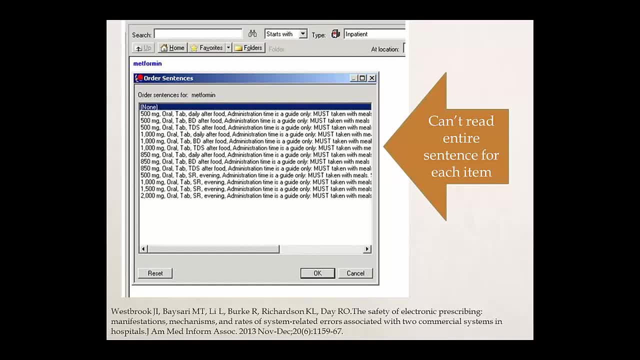 much easier for the eye to read and the organization of this is just crazy. so you have to use this slider bar across the bottom to actually see everything. the and the name of the medication is only at the top. it's not in the sentence, so there's no name of a medication in here. it's really cognitively the. 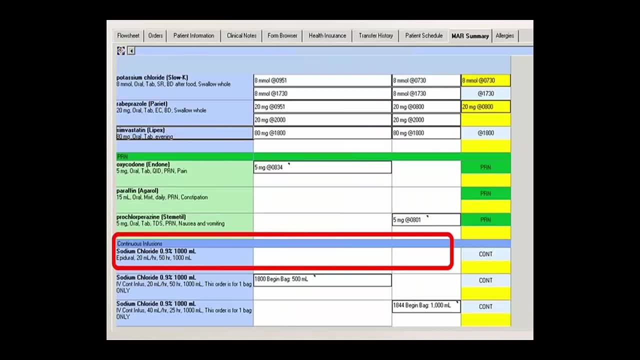 cognitive burden of this is huge. here's another example where the the this journal article gives a nice description of how some of these errors occurred. and down here, because of the proximity of of sodium chloride and the choice for an epidural route, this person was prescribed to receive a liter. 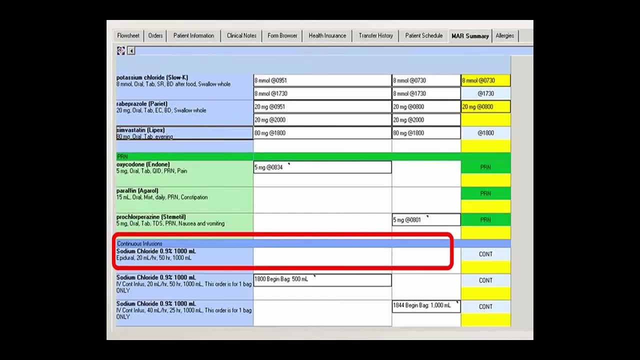 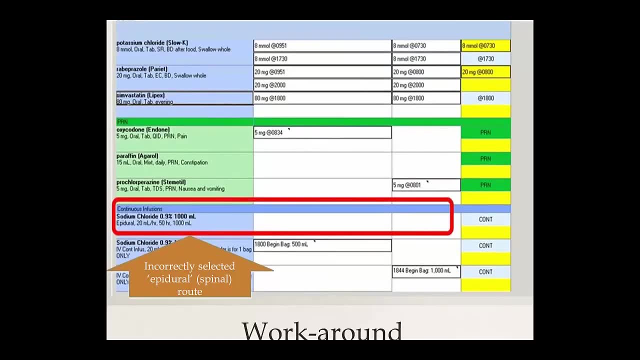 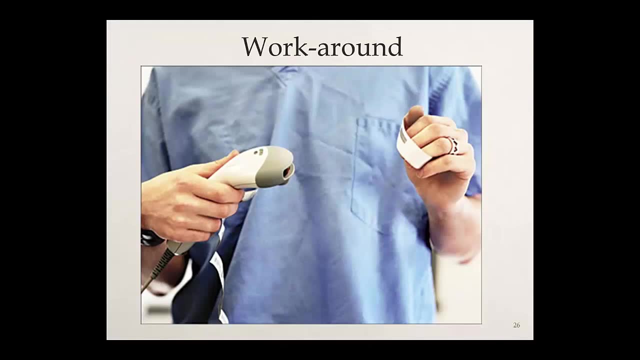 of sodium chloride epidurally ooch. so they selected the spinal root incorrectly but no alert came up. what was around there? I thought I had another one outside there- lots of evidence of nurses not liking the workflow that's imposed on them in using the computer system. so we've got evidence of nurses printing out all of the patient I showed. 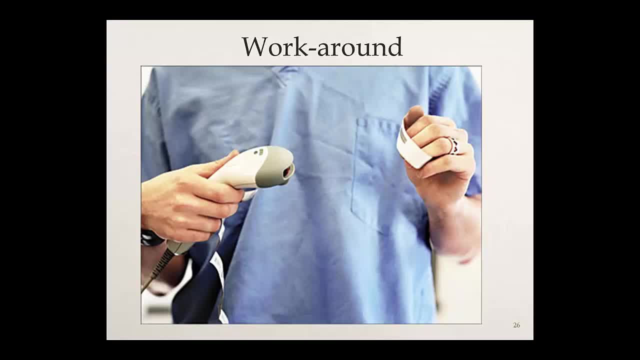 you the picture of the arm band and the spark code scanner. you go to the bedside and they're telling the patient to get to work, and then the patient just leaves and and then you touch the screen and you automatically collect these data. For various reasons, it either doesn't fit workflow, the machine might beep, 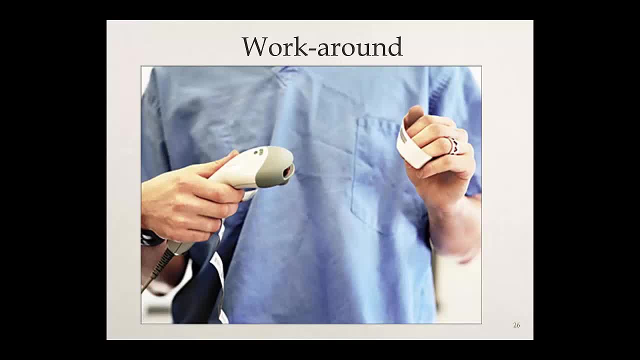 What do you do when you're on night shift? It's going to wake up the whole room, right. So lots of reasons why nurses are doing this. They're not doing it just to misbehave. They're doing it because there's something that's not matching their workflow. 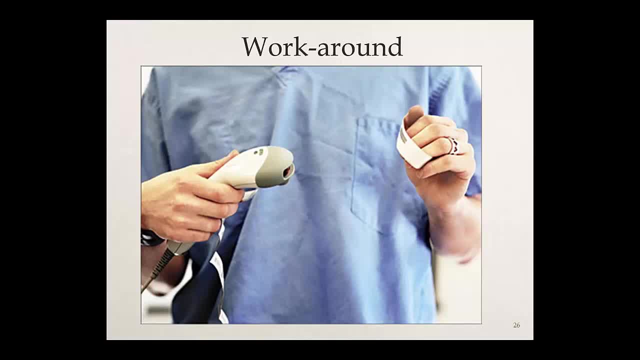 So they'll print out all of the patient labels, put them on a clipboard and carry out business as usual: Pull their meds out at the med part, take them to the room. But they've already done the barcode scanner and the time stamp, because they did that at the front desk. 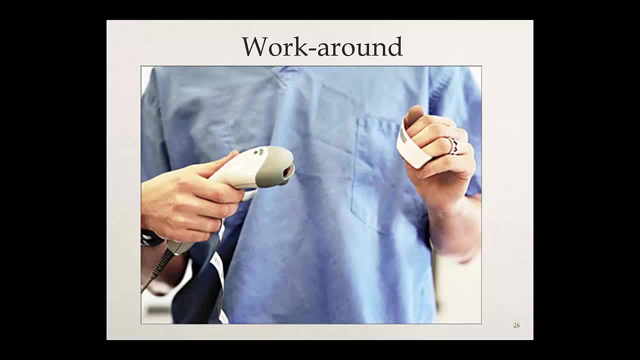 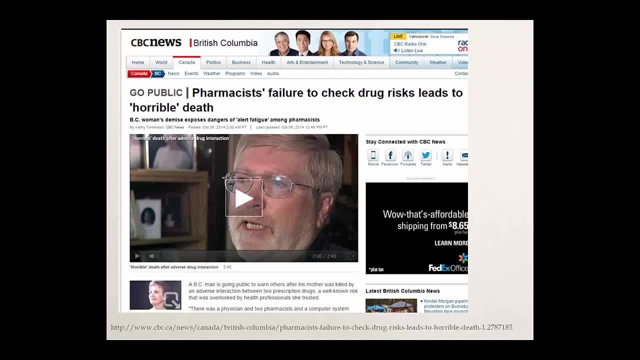 So figuring this out is really important. There's a great amount of evidence on this barcode- EMAR workarounds. Another example: last year in PharmaNet, pharmacists were permitted to turn off the alerts, So they had medication interaction drug alerts, and whoever designed PharmaNet let the pharmacists turn off the alert that there was going to be a serious drug interaction. 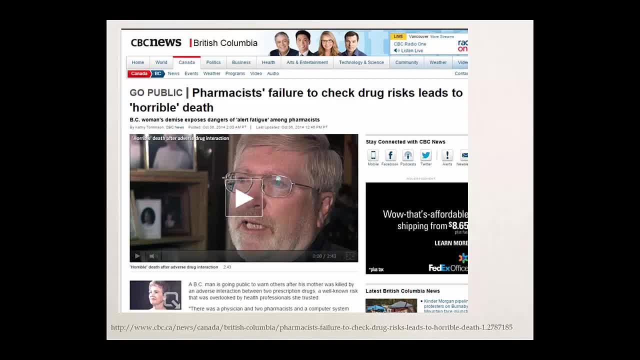 And so these two men turned off the alert and it ended up in a lady receiving two drugs. She, I think, was immunocompromised and she was given another medication that it put her at really really high risk for infection. 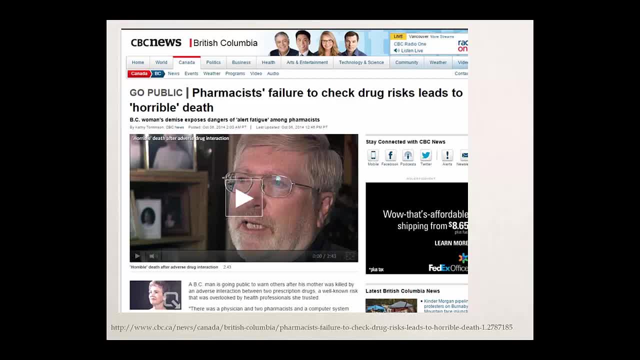 And she actually died of a serious infection in hospital up in the interior. Now, Fascinatingly, the pharmacists were penalized and so their licenses were suspended for about three months. Now we're looking at this from a patient safety perspective. 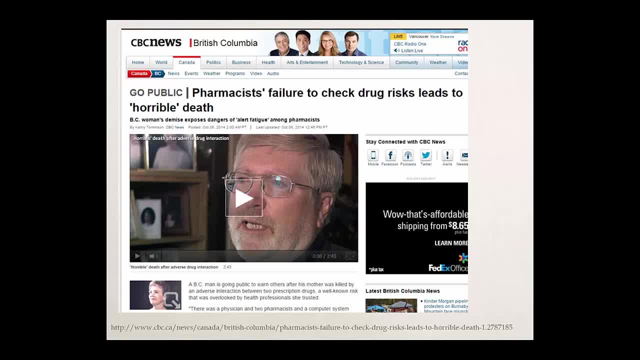 Instead of being in a blame and shame system, we need to understand where the system it's a system problem And I would argue that these people there should not have been a disabled function And there's Some recommendations coming out for different levels of disablement of alerts and we need to figure that out better in the field. 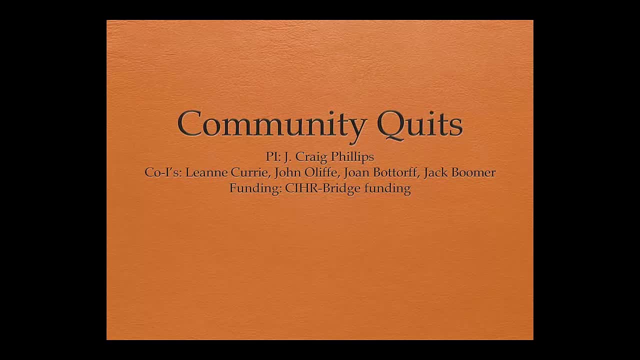 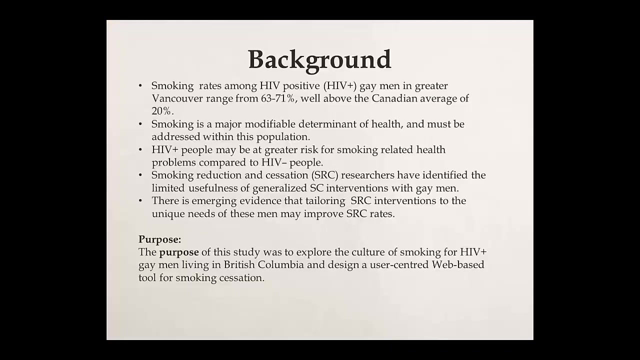 Now I'm going to talk briefly about a user-centered design project that I've been working on with Craig Phillips and we received some bridge funding. We're calling it Community Quits and it's for HIV-positive gay men, Because we men- in the Vancouver area, 63 to 71% of HIV-positive gay men- smoke cigarettes. 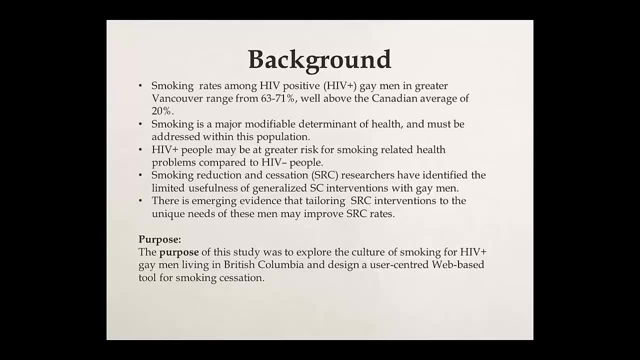 And this is a huge deviation from the Canadian average of 20%. We know that smoking's a major modifiable determinant of health and must be addressed in this population. There's actually some evidence coming out That HIV-positive people who smoke have worse health outcomes. 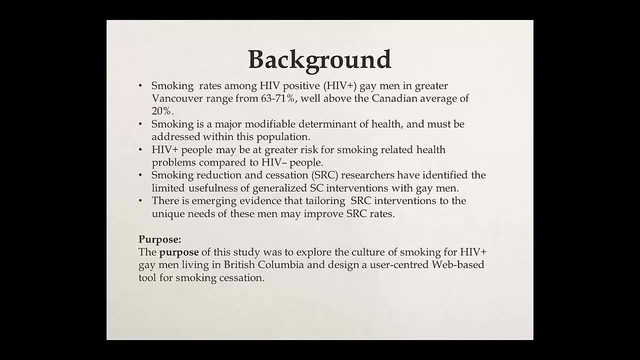 So it actually affects their immune system- Not surprising. So we've been looking at designing a smoking cessation tool that's specifically targeted to HIV-positive gay men. It hasn't- These haven't been Designed yet. So we were wanting to look at the culture of smoking and design a user-centered, web-based tool for smoking cessation. 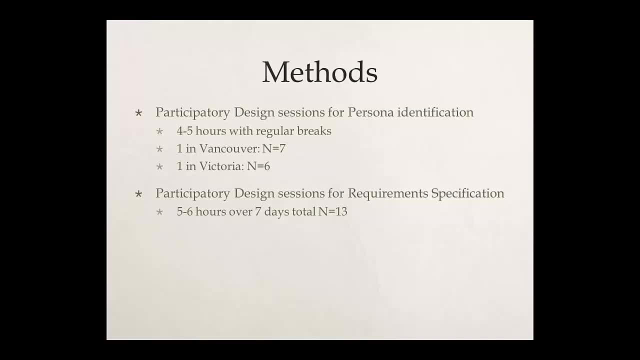 We conducted two sessions of participatory design. The first one was to identify personas and we had two four or five-hour day-long workshops to identify personas, and I'm going to show you what we did with that. And then we had 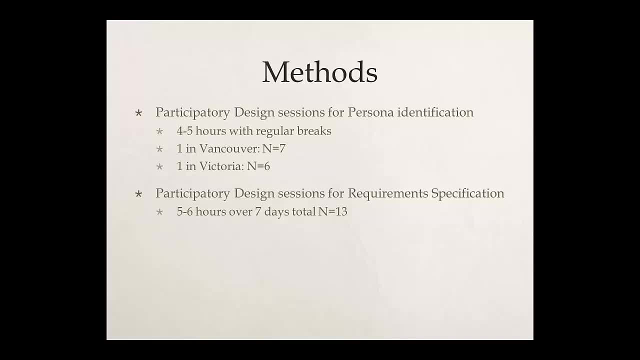 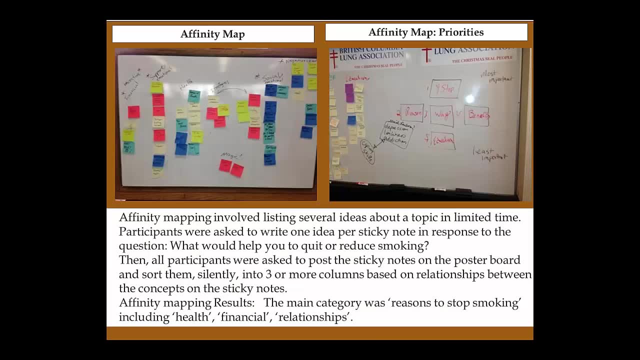 We had a total of seven days of participatory design for requirement specification. So what we? The first thing we did was a thing called affinity mapping. So we asked people to sit at a table and write down the things about smoking that they can think of. 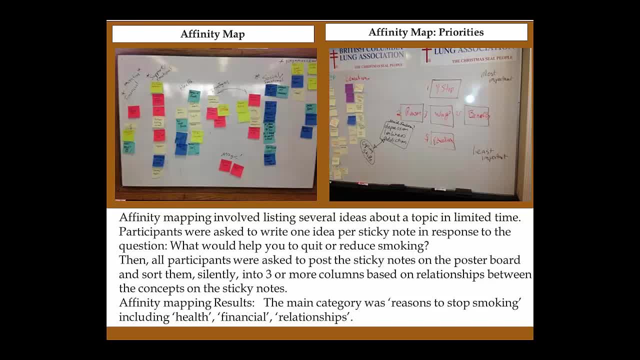 So write one thing on a post-it note. Then, silently and again, these were groups of seven, six or seven. Silently, they had to go to the sticky board. Silently, they had to go to the sticky board. 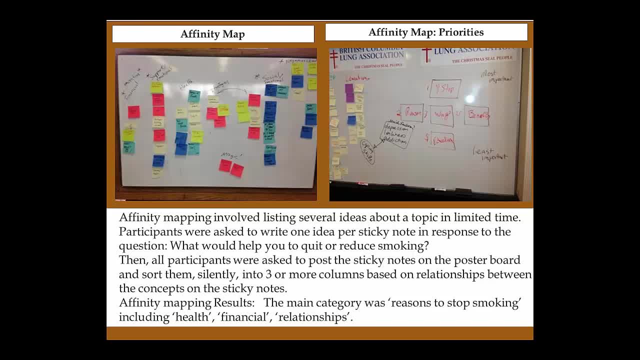 and put and organize them. They weren't allowed to speak, So we were using a process called game storming, where we were trying to make it a playful environment so that it sets aside your business head. Instead, we're making it playful. That theoretically allows for more creativity. 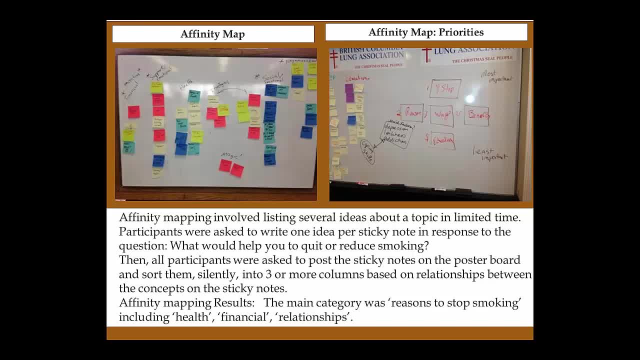 and it prevents people from second-guessing what their right answer should be. We then held a round-robin in the group to ask for priorities for the affinity mapping And the main category that. So this is thinking about: what information would you put on a website? 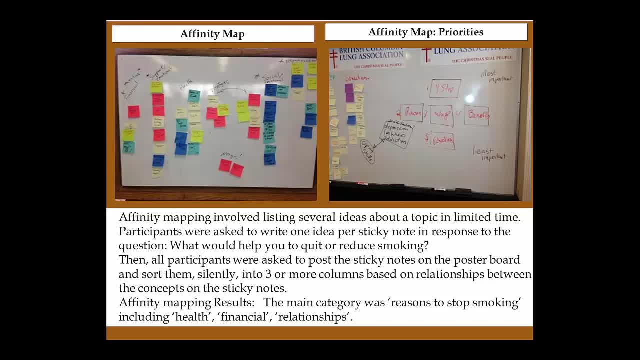 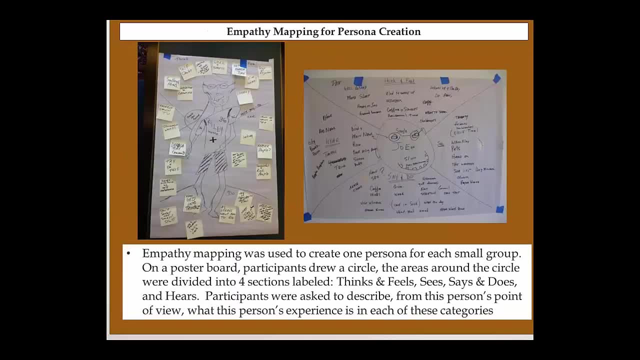 and how would you prioritize it? So the main categories were reasons to stop smoking, including health, financial and relationships. We then did something called empathy mapping, And this is- This is a game- where we had smaller groups of people- three or four people. 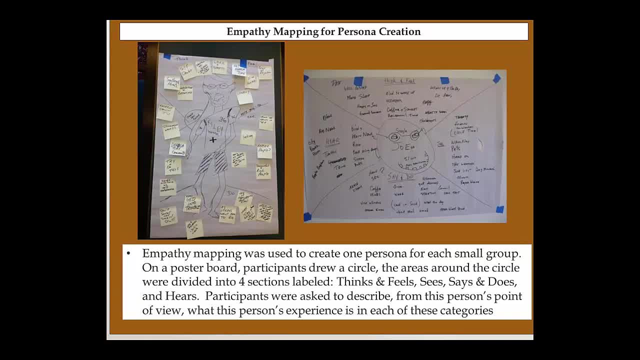 So each of the groups created two empathy maps And we used these to identify the typical HIV-positive gay guy who would be using a smoking cessation software. We let the groups, We walked around and kind of coached them into how to do it, And one of the groups 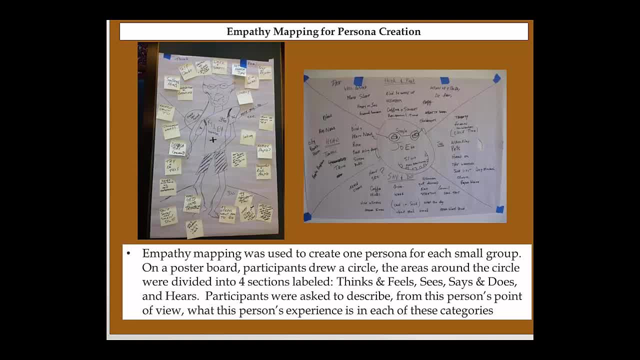 came up with this character called Riley Homo And we have different characteristics of him. We used this empathy mapping here for most of them. We asked them: what do you think and feel, What do you hear, What do you say and do? 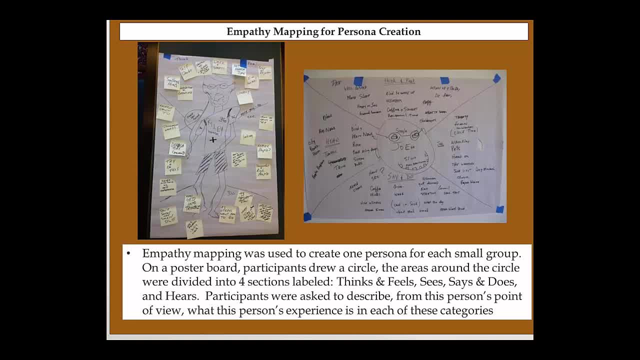 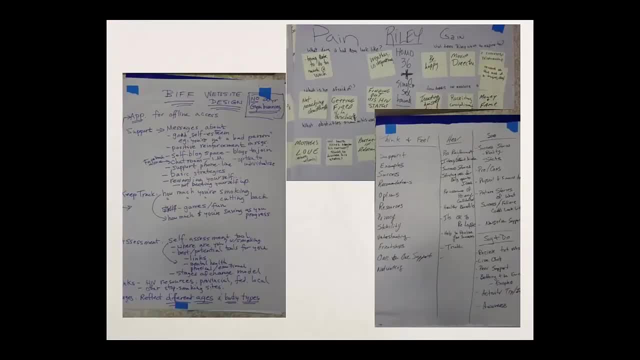 And what do you see? So, with all those, And then in the center of the characteristics of the person, We also asked them to then kind of go into: what do you feel? What do you hear, What do you see? What do you see? 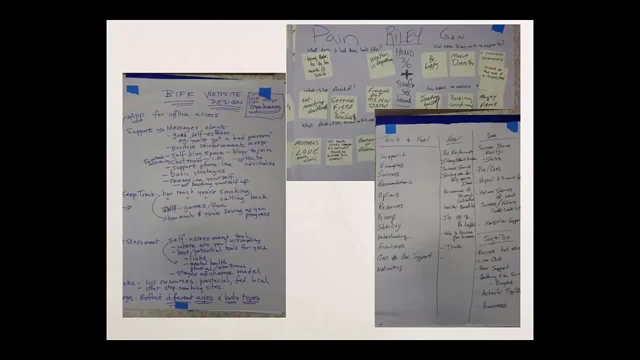 And then kind of tie that in- How do you think about what you are feeling, How do you feel- And then kind of tie that in go into the website design. We had them do this pain and gain activity and we then summarized all the think and hear and see and say We then created some. 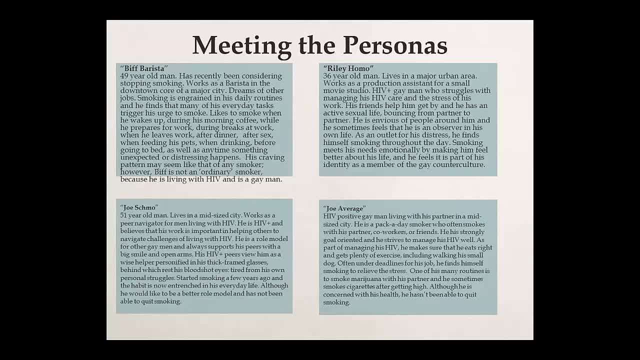 personas. So this is a persona. This is the character that you would give to your designer. that is the typical person who would be using this system. So each of the groups named their persona. The first one was called Biff Barista. He's a. 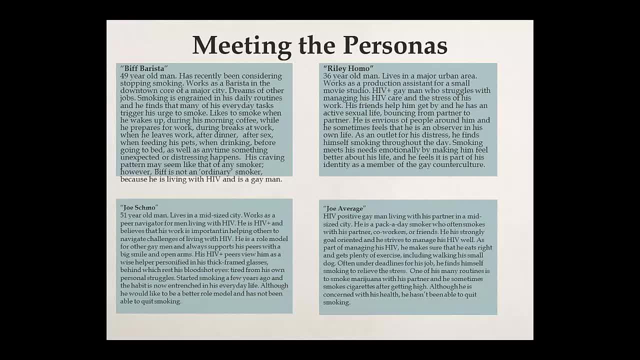 49 year old man has been considering stopping smoking. works as a barista in the downtown core of a major city, dreams of other jobs. smoking is ingrained in his daily routines and he finds many of his everyday tasks trigger his urge to. 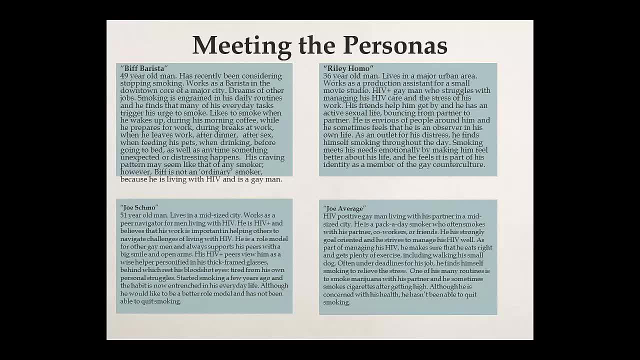 smoke Likes to smoke when he wakes up during morning coffee, while he prepares for work, during breaks at work, when he leaves work after dinner, after sex, when feeding his pets, when drinking before going to bed, as well as any time something unexpected or distressing happens. I'd say this: 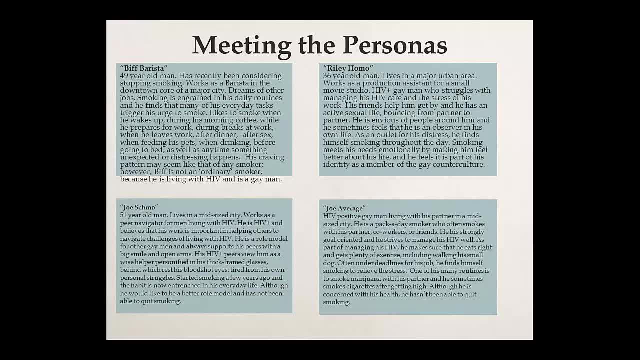 person's addiction scale might be kind of high. He's his craving pattern may seem like that of any smoker. however, he's not an ordinary smoker because he's living with HIV and is a gay man. I'm not going to go into detail on the 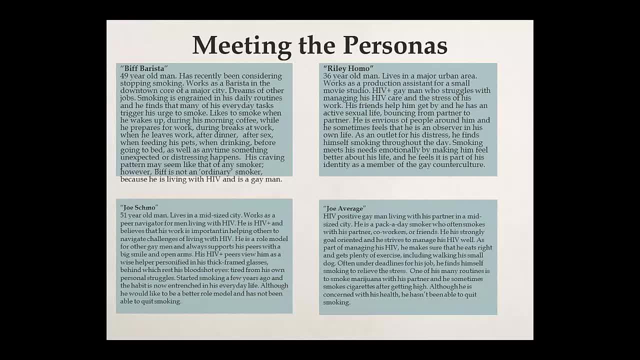 others, but they were all quite similar. We actually did a persona validation episode in our second, in our second visit with the group, and one of the younger guys was kind of angry that all these are 50 year olds We want. so we've created a new persona that's a 25 year. 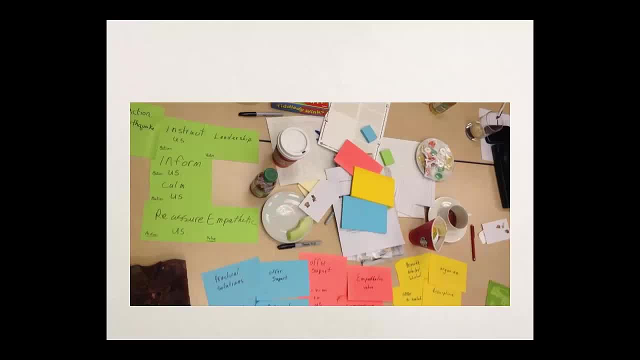 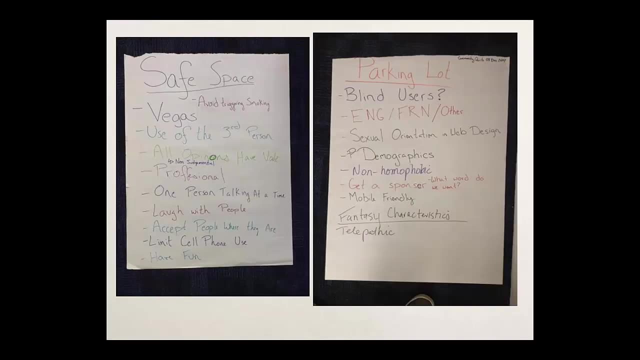 old. This is our participatory design. what it looks like, It's a big mess and you have to be able to manage that kind of chaos if you're going to do this kind of work. We then, in our second phase of participatory designs, we had a larger 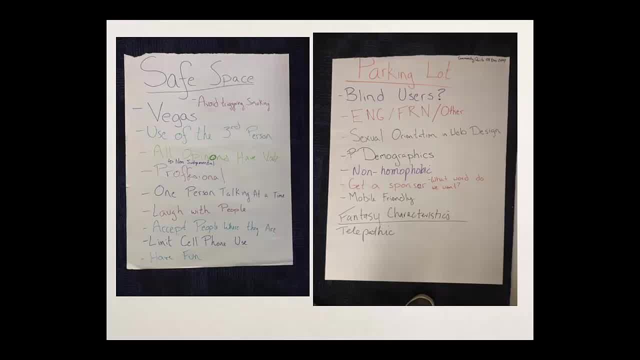 group of people For both of these sessions. we create a safe space dialogue and then we have a parking lot- Stuff people might want to mention but we don't want them to kind of go down that path and really hijack the conversation. So we have a parking lot in the safe space. We say it's like Vegas. 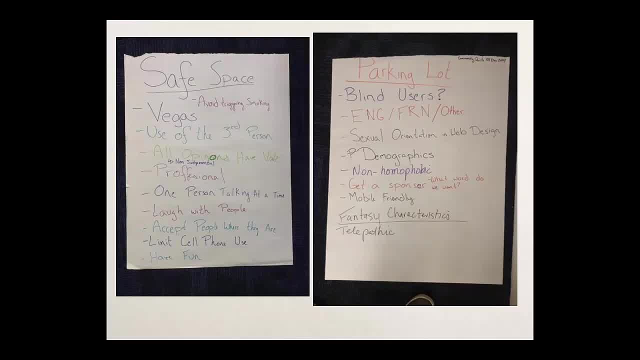 in this room So you guys might know each other from your community activities. but everything that's in this room stays in this room. Of course, we have consent when we're before. anybody participates in this, One person talking at a time. We 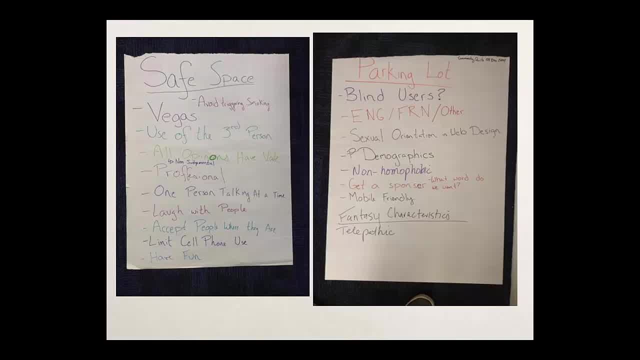 want to laugh with people, So we create this safe space agenda with the community at the very outbreak of this starting. It's excellent, It's it's super, super fun. It helps you manage a big group, especially this group. We had 13 people. 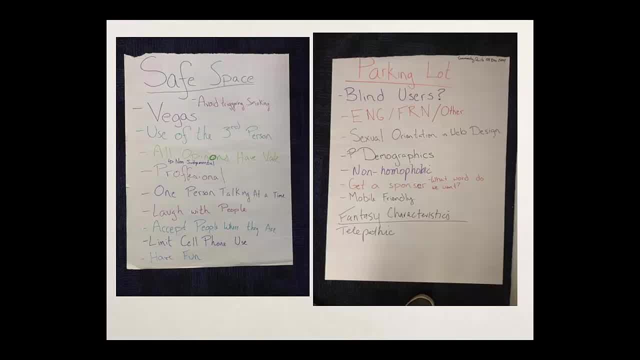 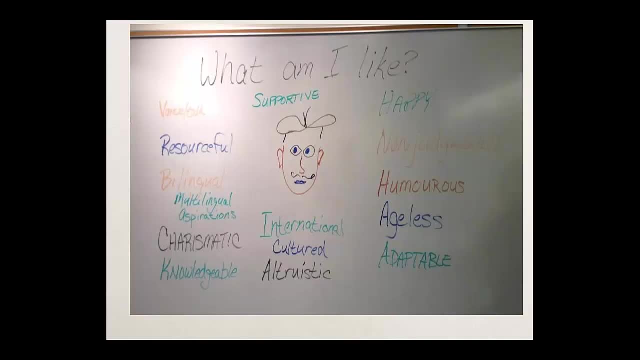 in it and it was. sometimes there would be some challenging behavior, So we could bring it back to one person talking at a time. Please laugh with people, not at people, That kind of thing. We did an activity called Product Pinocchio and we 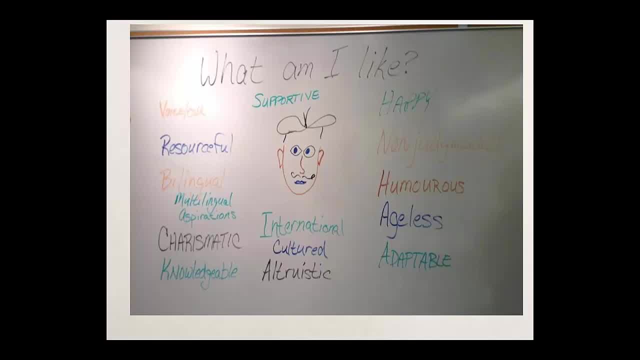 asked people to give us the characteristics of this software, So this is what they came up with. They actually named him. His name is peer support because he's going to be a peer support tool. You can see how optimistic he's. he's got some sort of a voice they want. He's resourceful. He's bilingual- We did 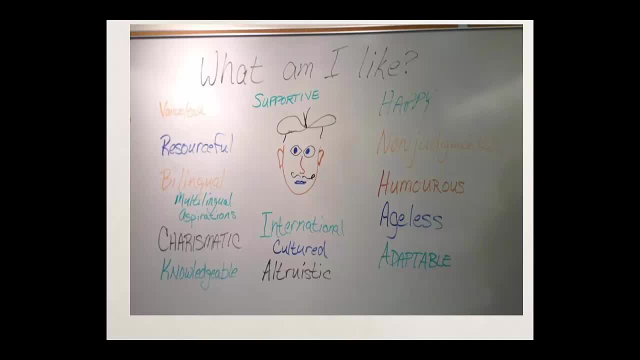 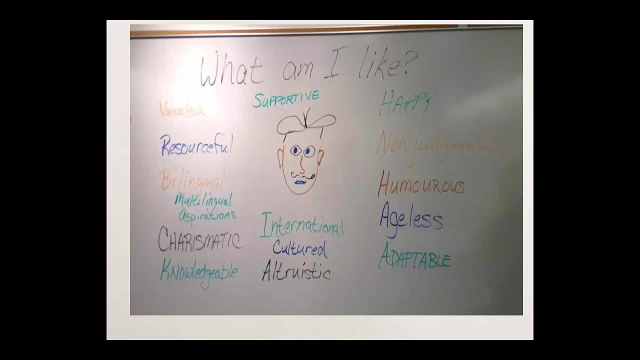 international, cultured and altruistic. He's happy, non-judgmental, humorous, ageless and adaptable. So these are all very aspirational And when you're actually working with a designer, these are the kind of words that you want to. 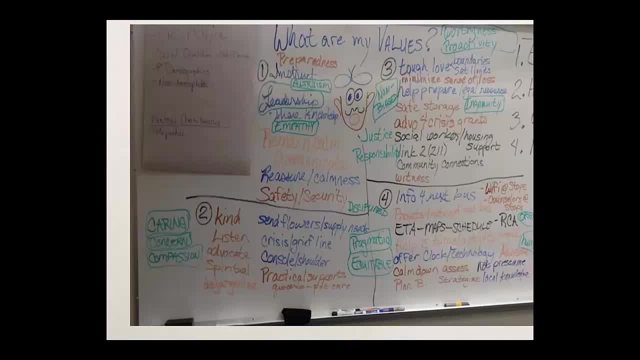 kind of anchor around. How am I going to design this thing? We then did a value mapping activity And we used a number of different challenging scenarios, and what were the values were enacted in those, and we we came up with a list of these characteristics. 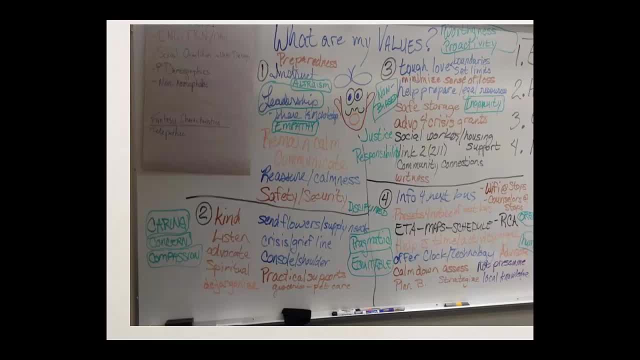 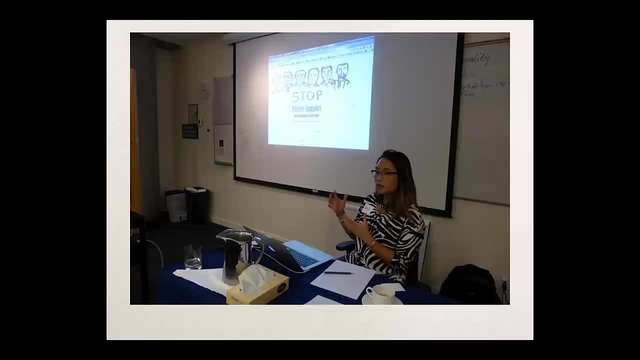 pragmatic, equitable, caring, concern, compassion. and then we found out what's the community we also. this is Charlene Ronquillo, who's a PhD student here and who was working with us as a research assistant on this. we used a wire framing software and Charlene created a fake website- just the front end of it- using a. 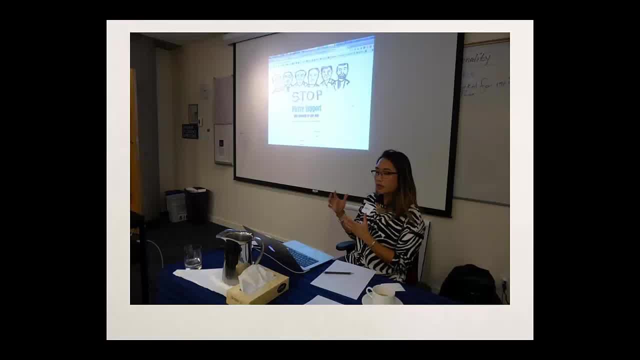 software product called Aixure. we had all of the guys and I don't have a photo of them, but there was 13 guys, with some with iPhones, some with iPads, some with laptops, who were all clicking as she was designing. it was mayhem, but really. 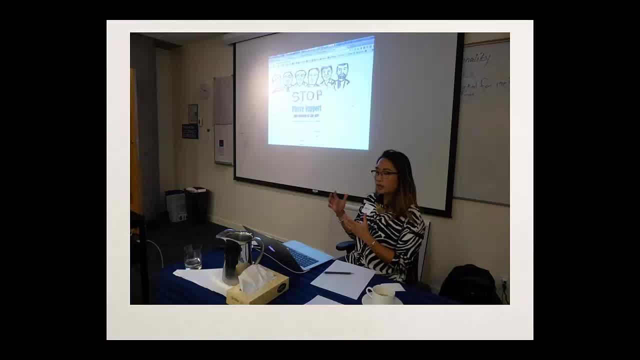 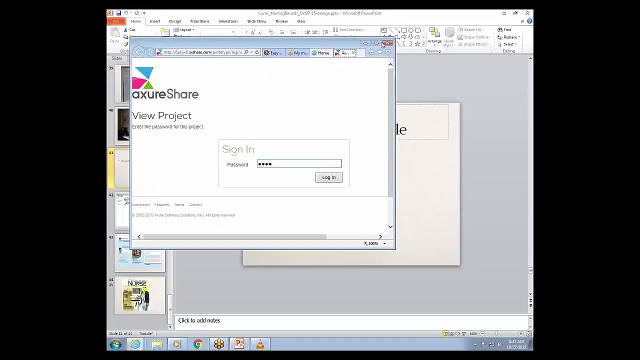 exciting. they felt so engaged and they felt like we were making a difference. and that's what we did here in New York City and we were able to gain like we designed this. I'm going to quickly show you the product. I'm just going to show 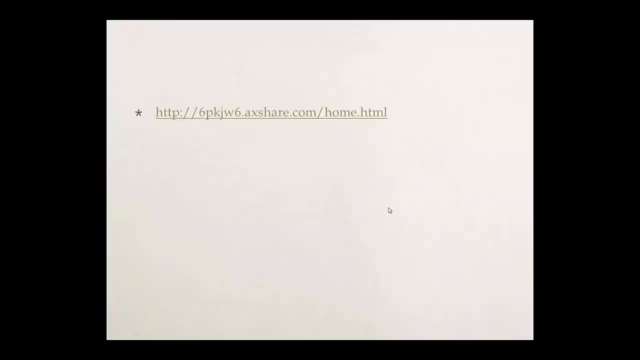 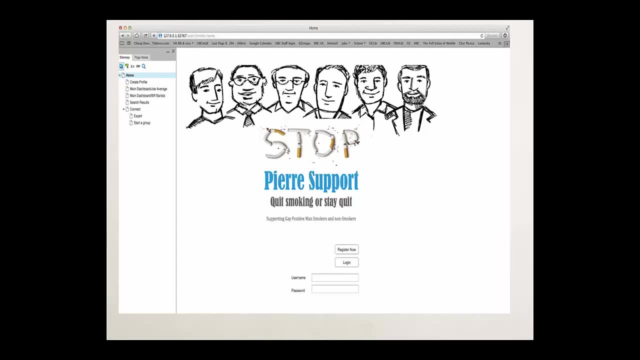 you the screenshots of it then. So we created this peer support and it's a clickable site and the guys in our project were clicking through it and we were. we didn't have quite enough time in our study and you know, for our next study we'll plan much more time where 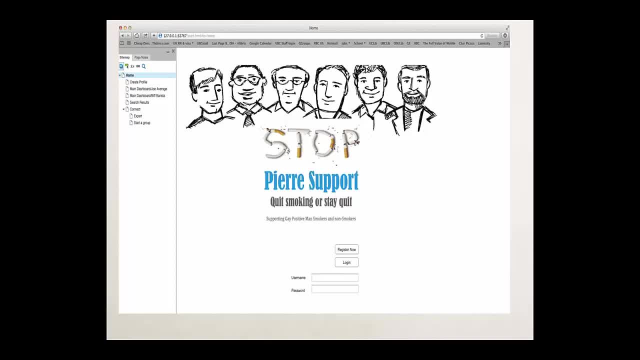 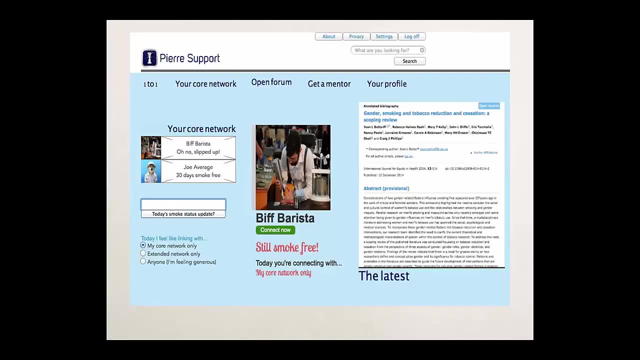 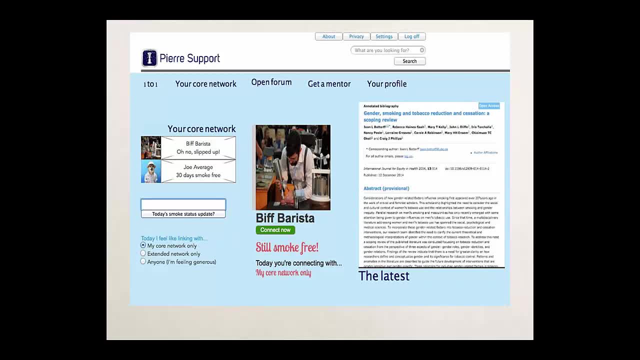 data that we have, but we're sharing it. There are some things I wanted to show in terms of how it works. So both personal designs, like the one in the above slide that I showed you and the one we showed you already- they are instead created using κoplay or. 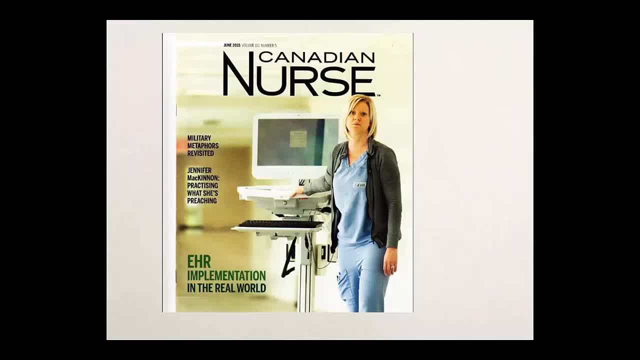 theressed-control method and the closing part is almost the same, So these are different. this cover of the Canadian nurse- Yeah, what'd you think about it? She looks. yeah, so my goal in life is to help design systems that are going to be usable for. 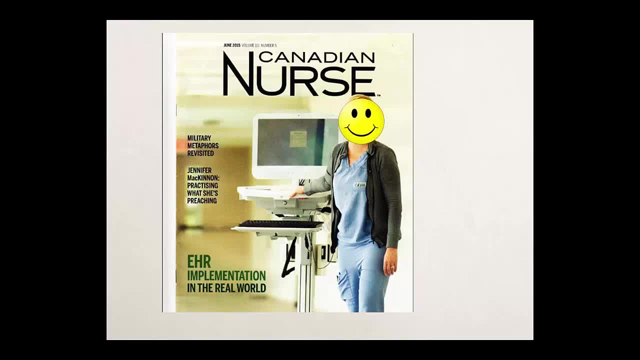 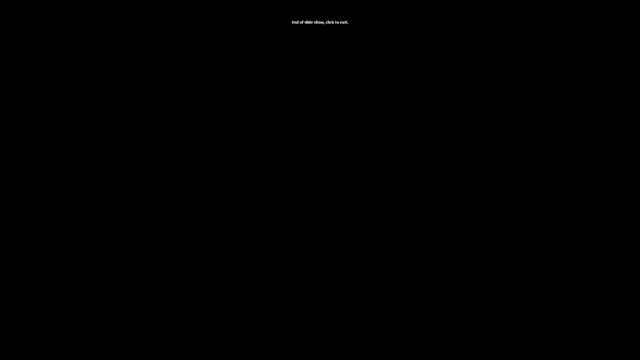 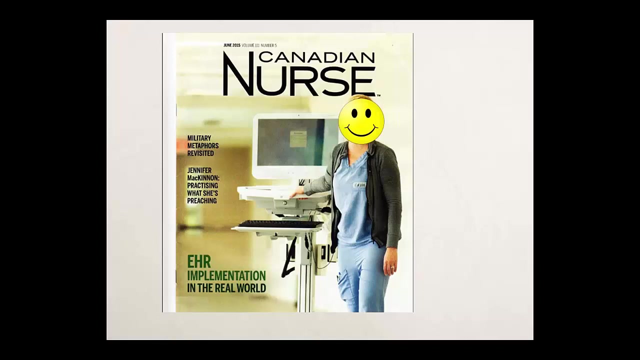 clinicians and for patients, so that we don't have this frustration and anxiety in and bringing the clinician into the design process. It's crucial and we have to figure out how to do it better. Thank you, Any questions? So, business best practice for software design. Did you guys online hear the? 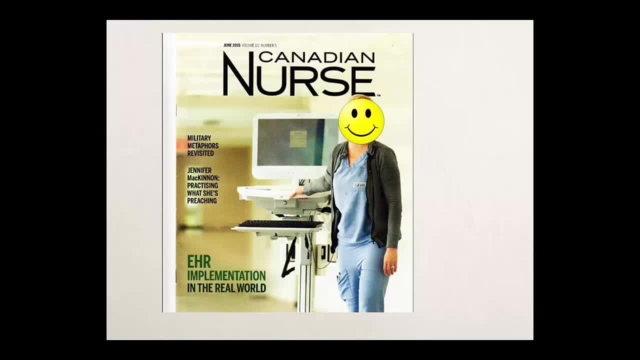 hear the question. I'm presuming you did, because the audio looked like it's pretty good there. So the business best practice is you would never launch something without getting end-user feedback early on. What's happened in software design? the whole process has matured over time. 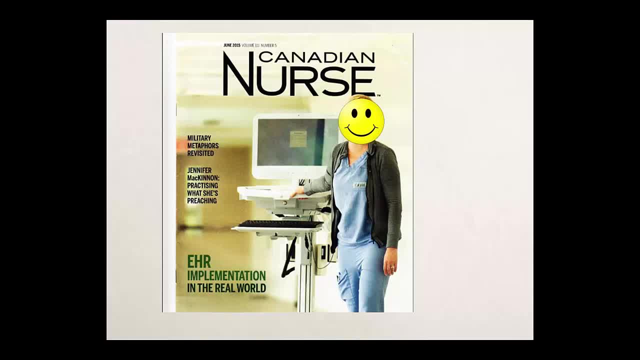 and people have thought that well, those are end-users, they're not experts and I'm the expert, So there's a power dynamic. What some groups are trying to push the agenda for, involving end-users in using like a wireframe or something that's clickable. 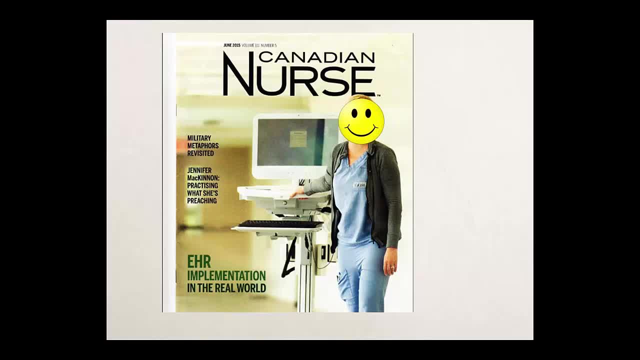 through very early on, before all of the hard core programming is done. We're a little bit about using the development site without doing prototyping before that, because you could actually take screenshots of the system, shove it into one of these wireframe things and drag stuff around. 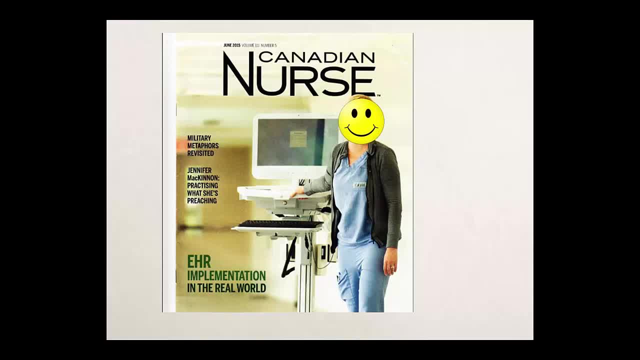 and drop it around The other stuff. you're relying on the the development team to who are the software programmers, to design what you tell them from, probably a paper prototype- hopefully at least paper and not just something verbal. So I'm working with PHSA right now to try and help them. 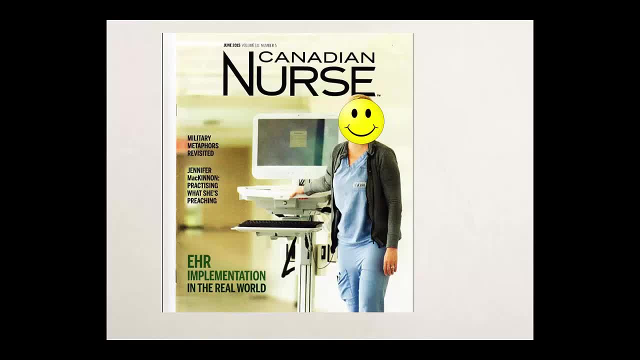 think about doing wireframing. earlier on I've talked to the CST leads to kind of give them a little bit of this talk, but they I don't know if that machine can be steered away from the traditional software development process in an. 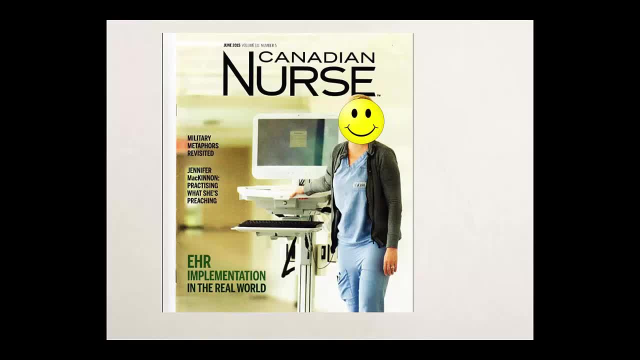 organization: Yes, Wendy, And he was using Agile? Yes, But he came up with this grounded theory that talks about reconciling perspectives and what happens with software developers when they're not entirely clear that they're having good communication with the client, and talked 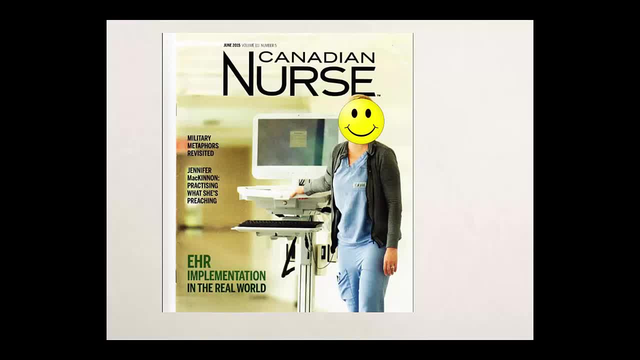 about things like bunkering, where they lock themselves in rooms and try to keep everybody away. Has anybody actually looked at what's happening more on the side of that Software development side with the user or purchaser interface? Absolutely So I mean, that's the team that usually needs to have some lead. 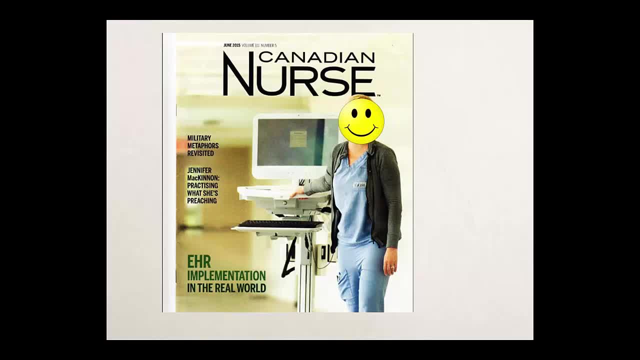 organizational leadership to facilitate that communication and building that trust. But that bunkering is classic, It's an us and them thing. So when you see a client, they're not so much a data scientist, they're actually a data scientist. They're. 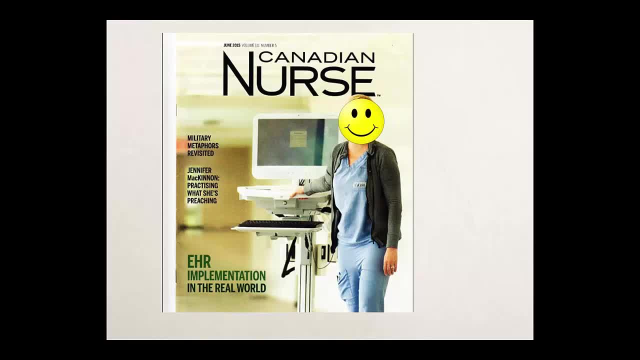 not a data scientist. They're just a data scientist for the team, So I think that's the point. So the literature that's coming out about organizational leadership and software design in healthcare is suggesting that the leader can bring those the geeks. 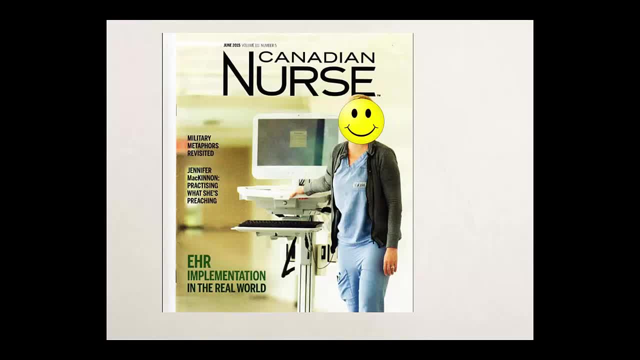 and the clinicians together and get a respectful and actually working together towards something. Part of that can be overcome when you have clinicians who have self-discipline and they're some formal training in clinical informatics, So they know the language right, They know what a use case is, They're not looking like a deer in the 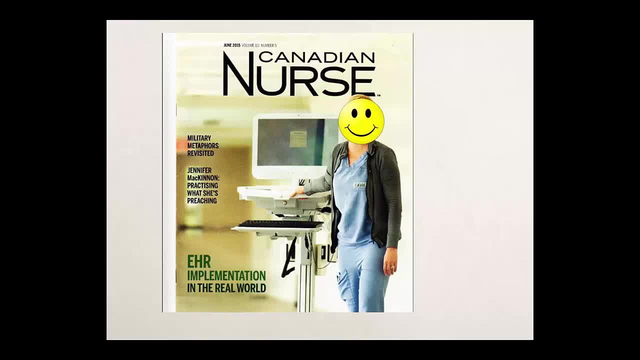 headlights when the software engineer says something, So the software engineer feels like they're responsible for all of that. So there is best practice and if you were the leadership talk last week, Betty De Silva talked about how she's trying to help her development team at PHSA actually adhere to best practice in 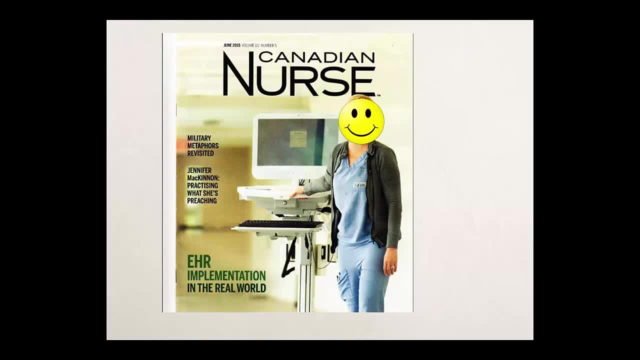 software design, Because it hasn't been invoked fully in healthcare and we need to get there. I just had a quick question about how, about cost, and how does that play into number one on the GHR side of things? how do organizations go about costing these things out? and then how? 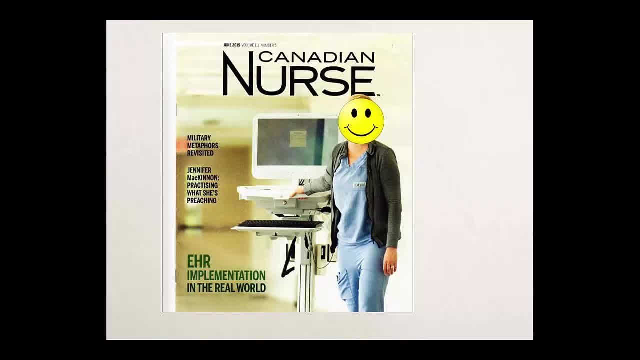 how do organizations go about costing these things out? and then how does that end up being an inhibitor to actually put it into practice? And then, on the other side, designing interventions for specific groups. What's it cost to design, for example, the website on smoking? What's the investment that you need to put in that process? 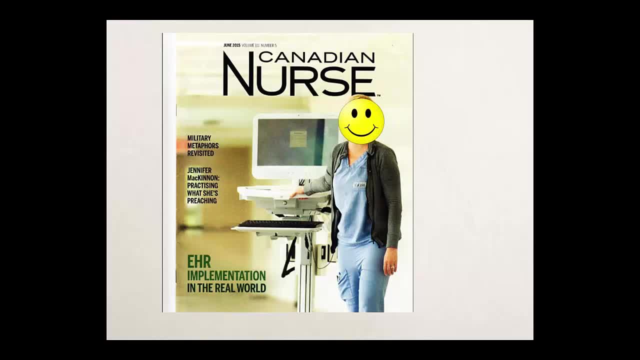 Well, it depends, and you know, if you were doing this as actually a product that is going to be marketable, as something that people are going to purchase. that's one thing. The return on investment is a big challenge. I don't think we know the answer fully right now, but if you're going to design something, 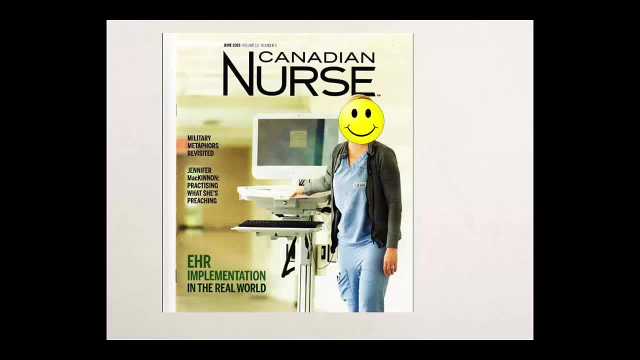 you're going to probably need at least a couple hundred thousand dollars to have a proper design team and to properly be figuring out the interventions. So in the context of the healthcare system. so the companies that have products will be, they have a ticket on it and then the organization needs to figure out how to. 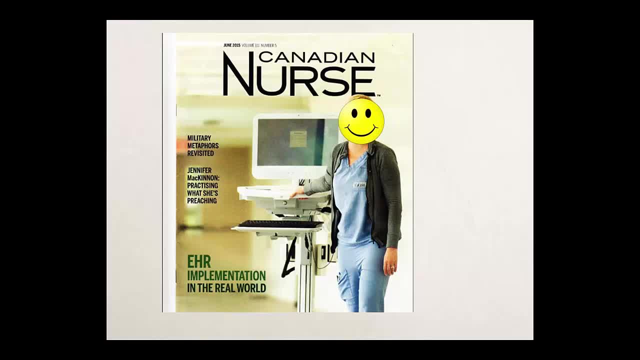 maximize the team to build that. So I know the price tag here is around 50 million, but that's actually pretty cheap considering. when I was in New York it was 50 million for two hospitals that I was at, and this is for 20 something hospitals. right, Yeah, but the key thing.